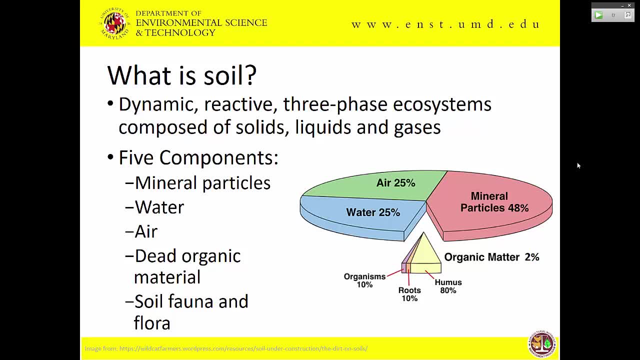 So that's about 50%. It's about the amount of pore space in the soil And, let's say, probably about two days after a big heavy rainfall, probably about 25% air, 25% water, so 50-50 air and water. 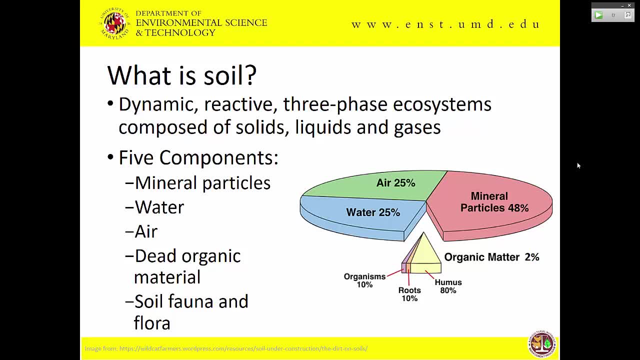 But it's going to depend right After a big rain, probably going to have a higher percent of the water, less air. versus days like today when it hasn't rained forever and it's been really hot, we're going to have a lot more air. So this one will change the ratios. 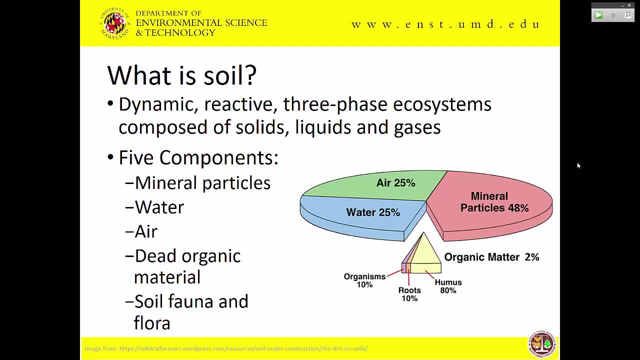 Then you have your organic matter. On average here in Maryland it's probably about 2%, but I've seen a whole range Fields that have a lot of organic matter added to them. I've seen up to 8% here in Maryland. 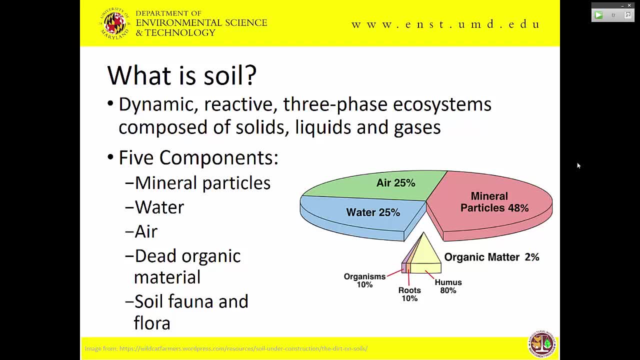 We've also seen a lot down in the 1% range for places that just use like chemical fertilizers- not necessarily the organic stuff as much. But then you also have to think about the different aspects of the organic matter: The living things, the dead things, the things that things exude, all kinds of fun stuff. 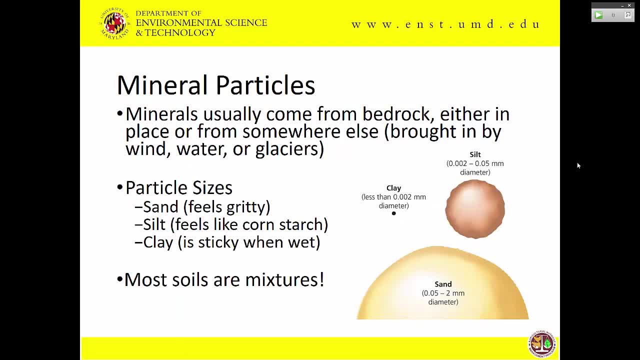 in there, So we'll go to the next slide. Okay, So we'll go over the five components separately. First up are the minerals, the sand, silt and clay. A lot of times these will come from the bedrock, particularly here in this area. 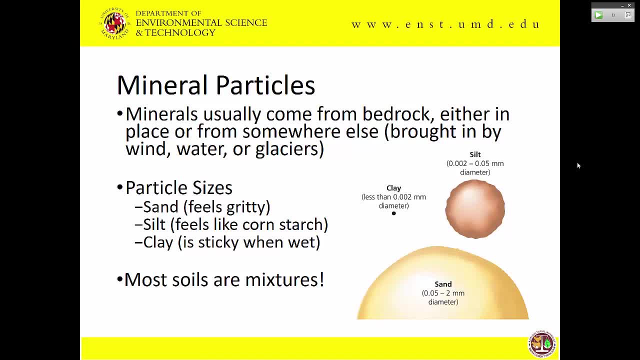 I've had too many glaciers recently, but they can be brought in by glaciers, can be brought in by sand or by wind, water, et cetera. They can be brought in from other places. Now, like I said, sand, silt and clay are the minerals we're talking about. 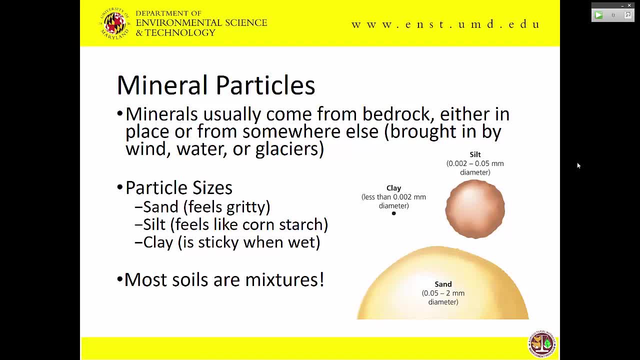 So sand, say You have all of them. You've all felt sand before. right, Everyone here has been to the beach. This is Maryland, right? You've all felt sand. Okay, It's very gritty, Say you blow up a sand particle to about this size. 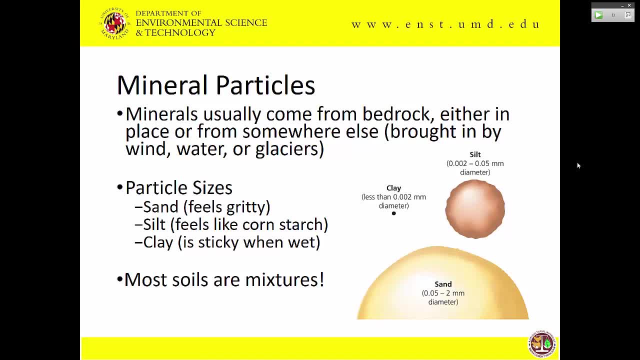 In comparison, silt would be about this size, and then this tiny little dot here would be a clay particle. Again, this is blown up and magnified a huge amount. Technically speaking, we actually do have size differences between these. Sand is 0.5 to 2 millimeters in diameter. 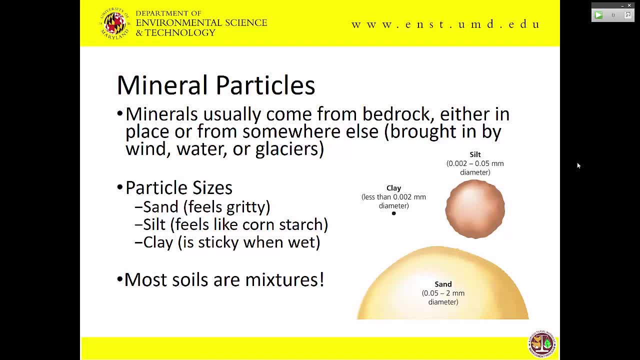 Remember, a millimeter is the total size, A millimeter is the tiny, tiny little thing on a ruler stick. Silt will be anywhere from 0.002 to 0.05 millimeters and clay will be anything less than 0.002 millimeters. 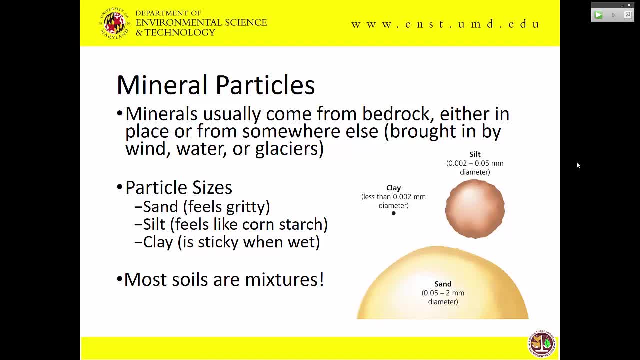 I can't remember if they would get that specific on the exam, but I figured I'm going to put that up there, just in case You never know. Patricia, she doesn't think so. Now I like to think of them as how you're feeling, because a lot of times people kind 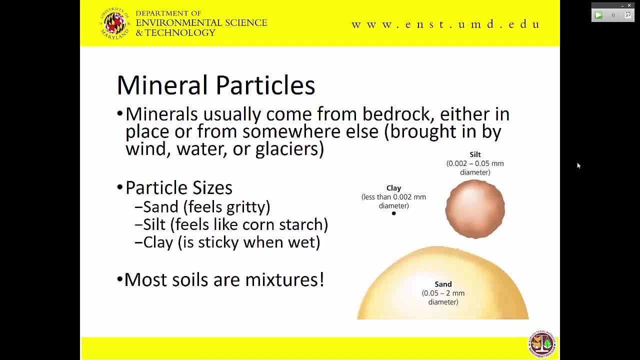 of just feel the soil, You can get an idea of what the texture is. just feeling it. Any kind of sand in your soil is going to feel real gritty. Again, you've all felt sand, so you know what I'm talking about, right? 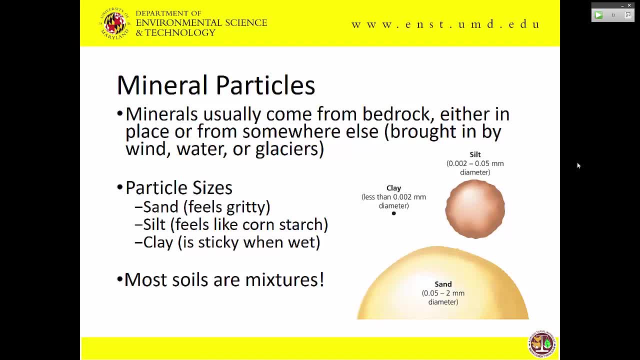 The silt. this is going to feel like cornstarch, a very smooth feeling. almost Anyone kind of ever played with cornstarch before It has a very smooth feeling to it. If you haven't go home, Check out some cornstarch. 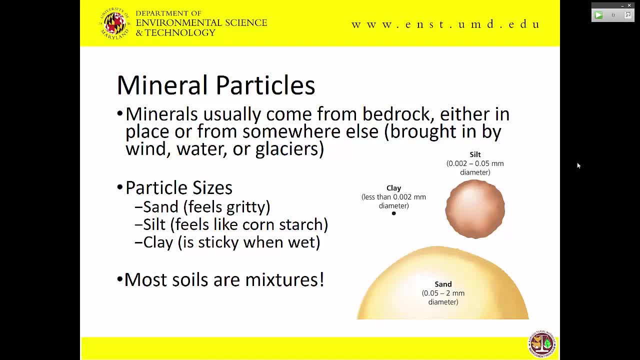 Clay- that's going to be that real sticky stuff when wet. Has anyone never played with clay or Play-Doh or anything? We all know what clay feels like. Now, a lot of soils are not going to be just one of these. 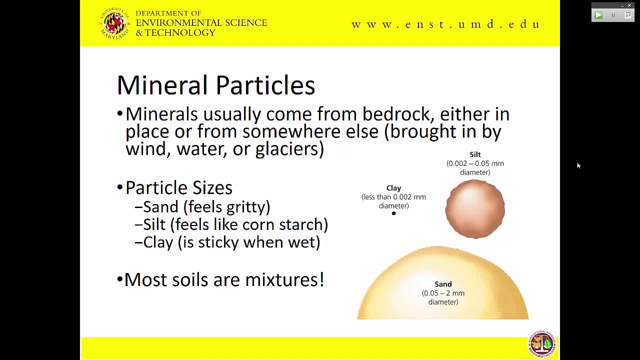 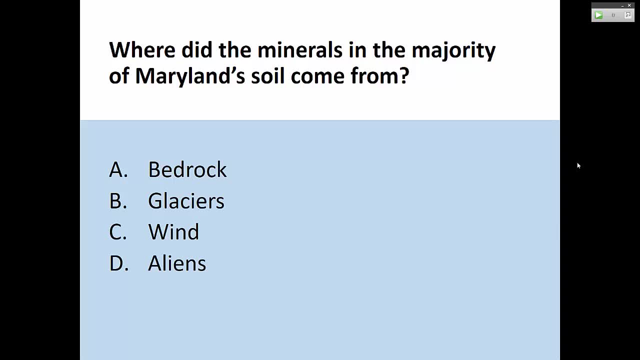 They're usually going to be all three of them, to some degree, Minerals in this area. I kind of spoiled it a little bit, but maybe you didn't all hear it. Where do they come from in this area? Go ahead, Let me get that started for you. 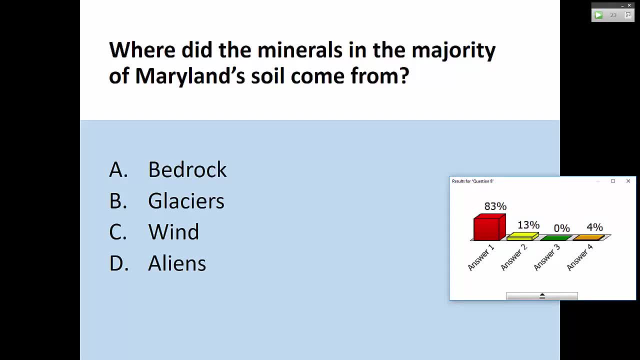 All right, You usually get a funny, funny person in here. It's not aliens, It is. It is actually bedrock here in Maryland Now, glaciers, places like upstate, New York, Minnesota et cetera. they had a more recent. 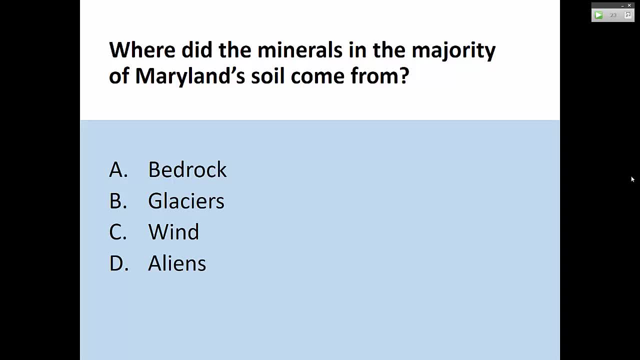 glaciation Down here in Maryland. it's been a very long time since we've had a glacier down this far. That's why we don't have many natural ponds or lakes, because all of them have eroded into streams and rivers at this point. 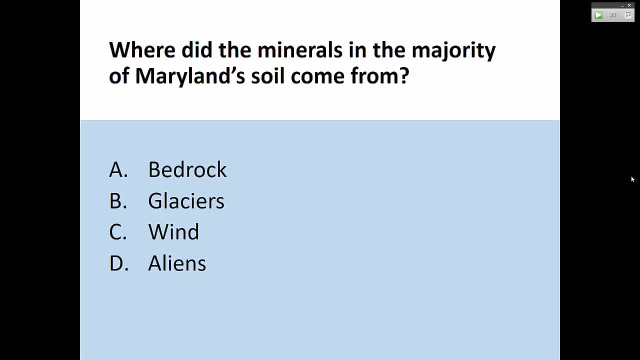 Most of it is going to be the bedrock. There are some areas where we might have had a little bit of luff, which is usually kind of silt, but it's mostly going to be bedrock here. So a term you need to know: soil texture. 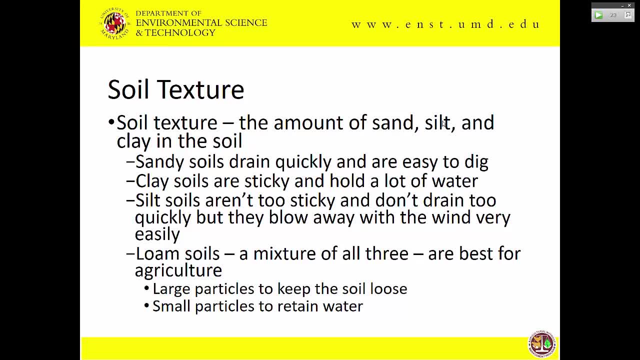 This is the amount of sand, silt and clay in a soil- One of those vocab words you're going to need to know. Now, all the different textures kind of have pros and cons. Sandy soil: they're going to drain quickly and they won't flood too much. 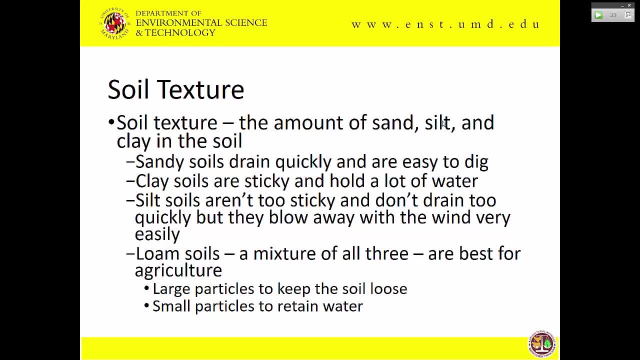 Really easy to dig, really easy to plant, but they can get droughty Right And your fields are suffering if you're not under irrigation because it's been so dry. Clay soils- they hold a lot more water, so they're going to need droughts, but they can. 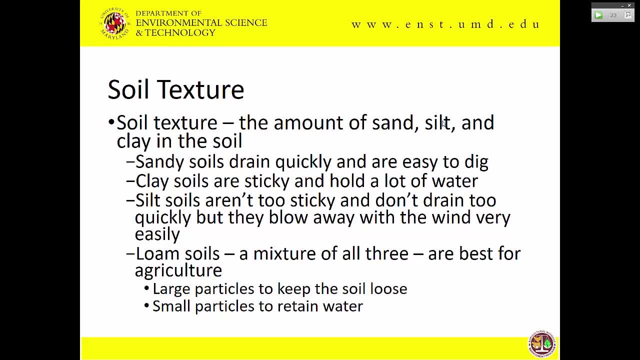 also be flood prone, so they can be problematic. They're also sticky and a lot harder to dig, especially if they're dry. Anyone have clay soils in your yard that they try to garden? Yeah, Not pleasant, Not a pleasant experience. 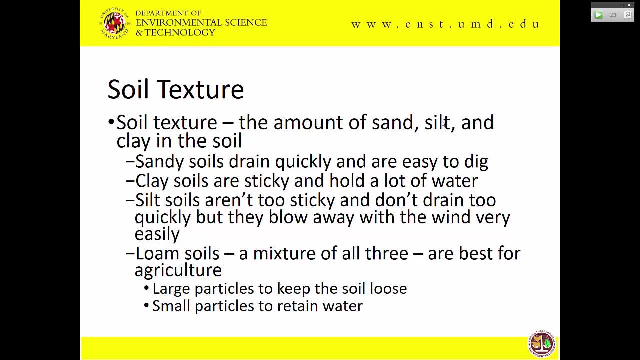 Silt soils are a little bit in between. They can hold a little bit more water than sand, not as much as the clay, So they don't have a lot of water, So they don't drain too quickly. but the problem with silts is they're the ones that 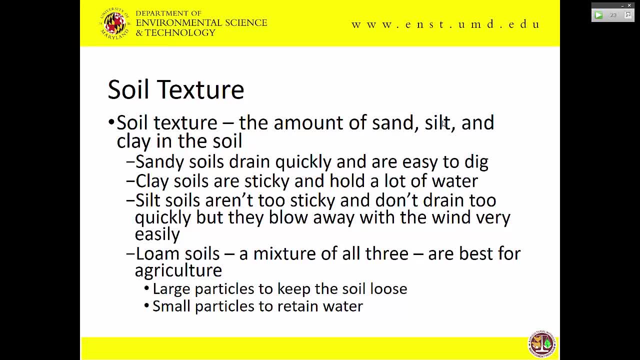 erode really easily. The clays tend to stick together so much that they don't erode as much, and the sands are heavier, So it's the silt. If you're going to get wind erosion or water erosion, a lot of times it's going to be the 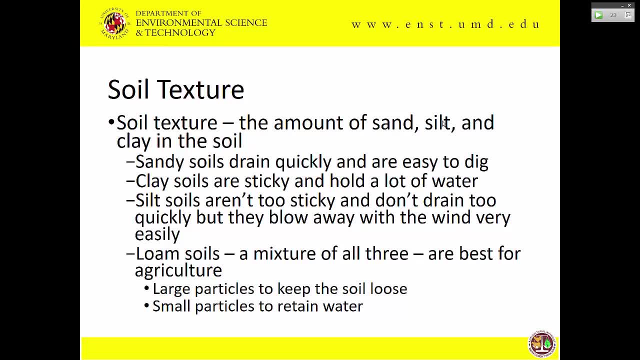 silt carried away. So, like I said, a lot of soils are a mixture. We call these loams. A loam soil is a mixture of all three and these are often the best kinds of soils that you want, Like if you're going to buy property and you know about soils you want to look for. 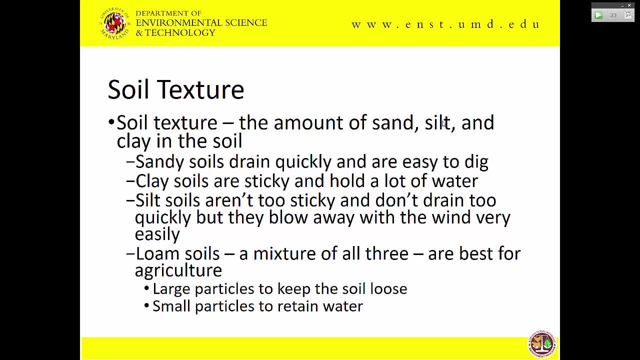 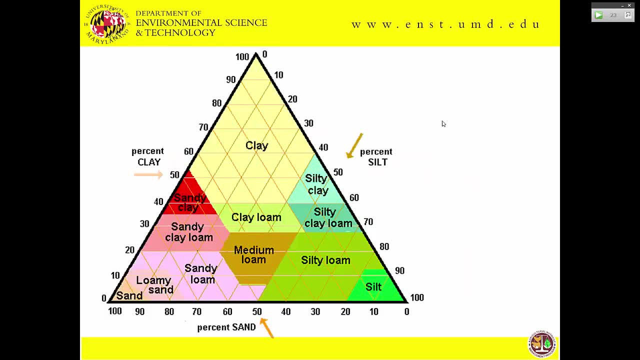 a loam soil. Large particles keep the soil loose so the roots can get down in. The small particles help keep that water. Now, this is what's called a soil textural triangle and, believe it or not, there are 12 types of soil. 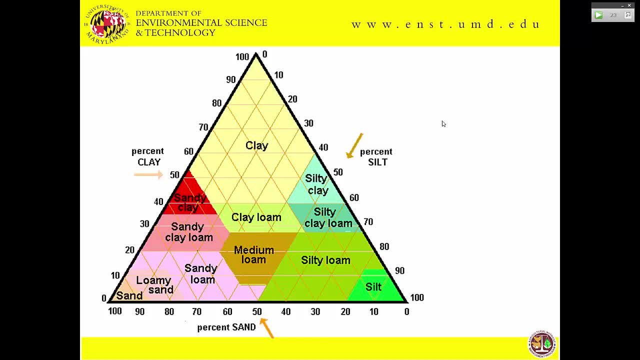 There's a clay, sandy clay, sandy clay, loam, clay loam, silty clay loam, silty clay, medium loam, sandy loam, loamy, sand sand, silty loam and silt. Who would have known? there are actually 12 types of soil. 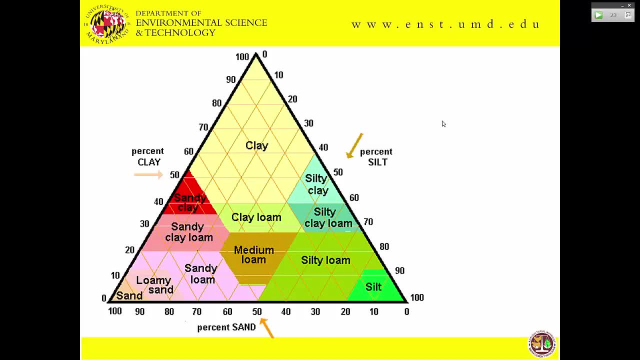 There are 12 types of soil. There are 12 types of soil textures. Now, what you do to read this is you figure out at least two of them, right? So, for instance, what is the texture of a soil with 30% clay and 50% sand? 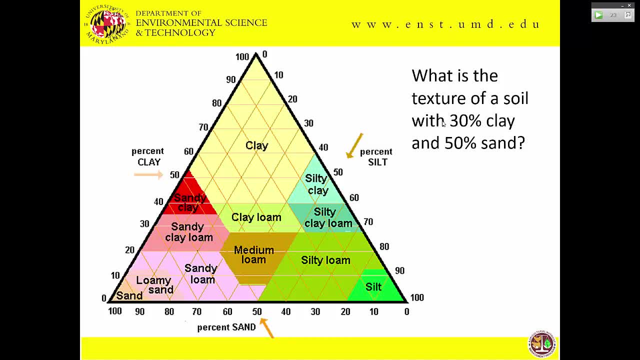 Well, the clay, the lines you want to follow are going this way. That's why the arrow points that way. So, if you have 50 or 30% clay, find that line, follow it out, Then sand. we're going to follow the lines going this way. 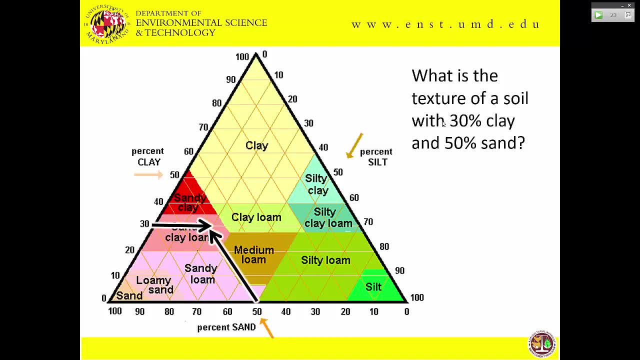 So you find 50% move up, got a sandy clay loam. It's actually kind of a simple way of finding out what texture you have. Now we also kind of call them different things. We've already used these terms a little bit. 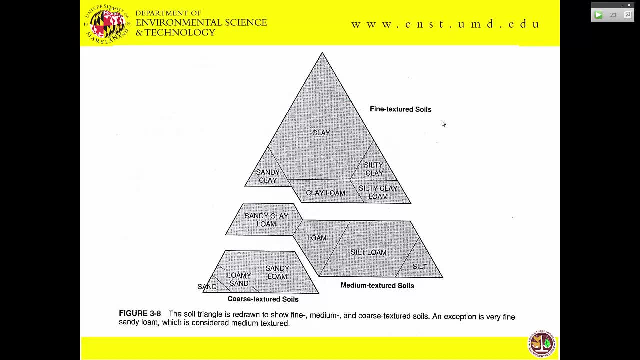 Fine textured. these are going to be the ones with more clay in them. The medium textured soils are going to have a nice mix: clay and sand and silt. The coarse textured soils are going to have a lot more sand. They're going to be more dominated by that. 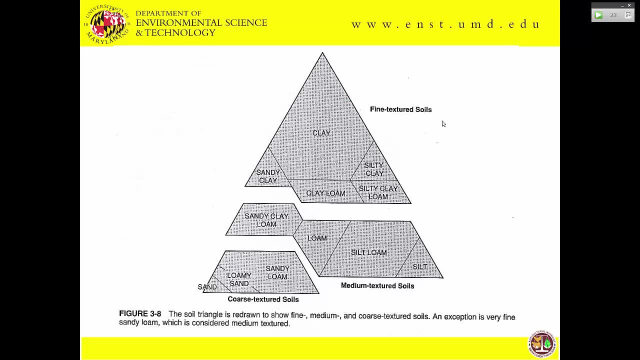 So when I say something like a coarse textured soil, I'm talking about something with sand. Okay, Then sand loamy, sand or the sandy loam, Finer textured soils. again, they're going to have a lot more clay. 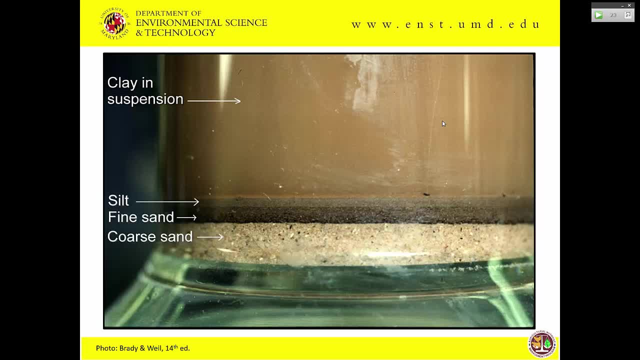 Now, an easy way to figure out what the percentages is is actually: just get a clump of soil, put it in a jar, shake it up real hard, Let it settle All the heavy stuff. the sands will settle out first. 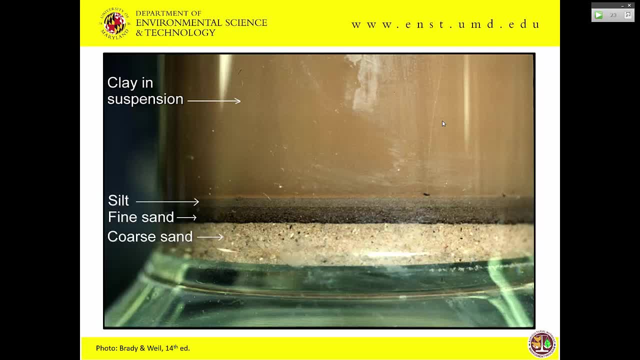 So you can see that this one actually has something called fine sand. It's this kind of darker brown layer. The silts usually take a little bit longer to settle out because they're not as big as the sand, but they're bigger than the clay. 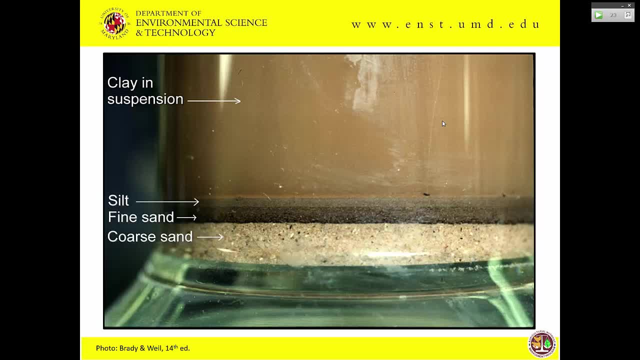 And then usually the clay. that can actually take like a full day, maybe even days, depending on how small it is in your soil, to settle out. But this is what the clay looks like in suspension. So then, if you just do, you can just measure these and do simple proportions. you can find out the percent that you have of each. 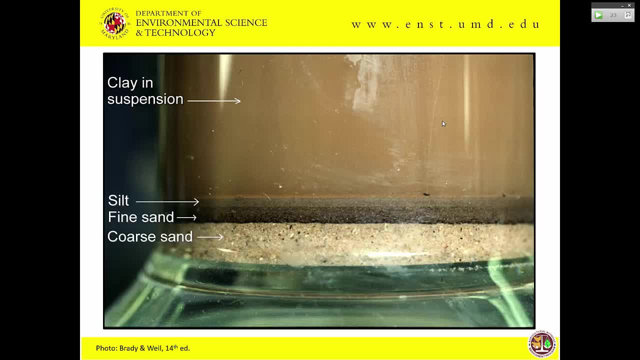 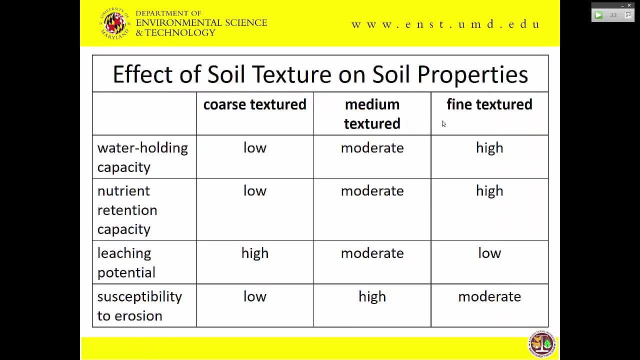 find out what kind of soil you really have. I know total nerd, Totally, have done this in my career. So why do we care? Because soil texture is important. Soil texture impacts how water moves through the soil, So water holding capacity, how much water they can hold. 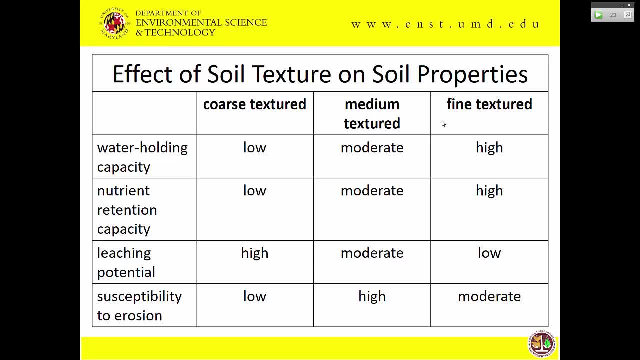 Coarse textured soils. this should be obvious. it's going to be low. They're not going to be able to hold as much water. Medium textured soils are going to be moderate. The fine textured soils: they act more like the sponge. 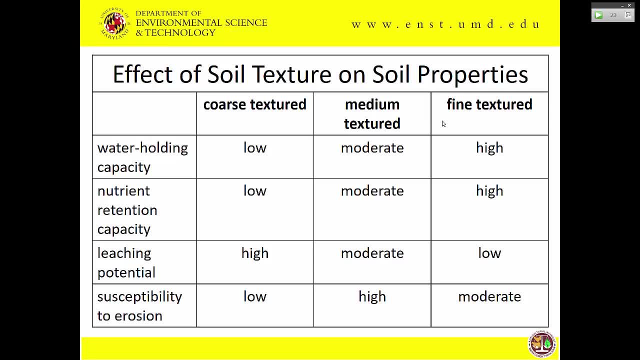 They grab that water and they hold on to it. The nutrient retention capacity is going to follow the same as the water holding capacity. Nutrients are going to be low in the coarse textured soils versus the fine textured soils- clays, for instance. 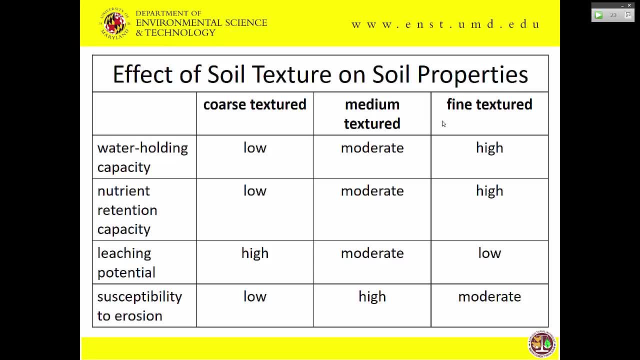 They like to hold on to things, especially those nutrients, So you're going to find more nutrients in the clays. Leaching potential is going to be kind of the opposite then, Because water can move fast and there's not many nutrients being held back by the soil. 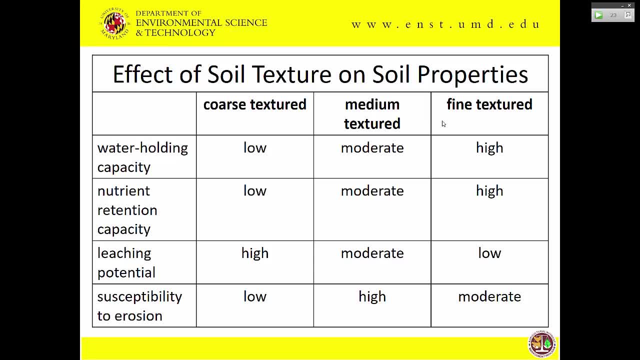 that means you're going to have high leaching capability Versus those fine textured soils. again, those clays. they like to latch on to it and hold on tight, So leaching will be a lot lower. The nutrients may be there. 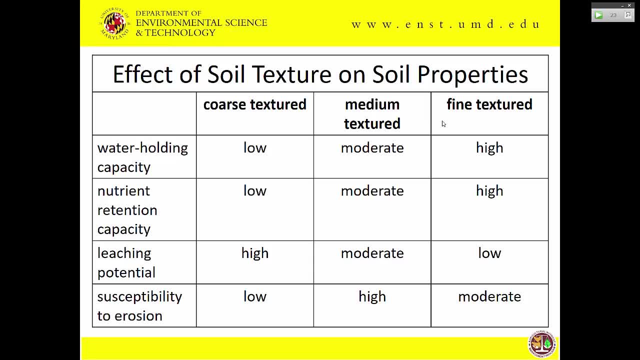 They're just not going to leave the system as easily. But the susceptibility to erosion. this is where things get a little different. It doesn't follow the high, medium, low categories. Again, the coarse texture is going to be low. 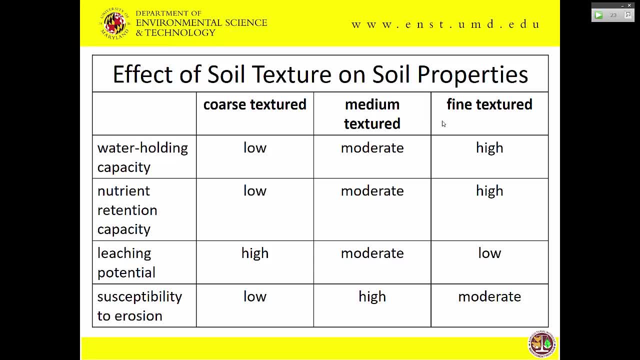 The sands are heavy, They're not easily carried off. The water has to be moving pretty quick Versus the medium texture that's the highest one there. Again, because there's silts, The clays stick together. The sands are too heavy, but the silts. 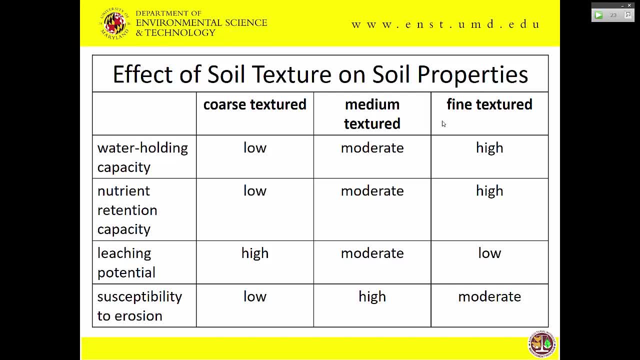 Those are the ones that like, if you ever see a dust storm, you're seeing more dust storms out in the west. Have you seen pictures of them recently going on YouTube and stuff? They're crazy. Those are mostly silts that are actually in the air. 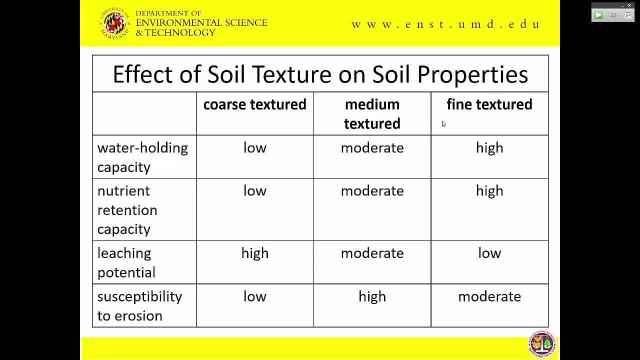 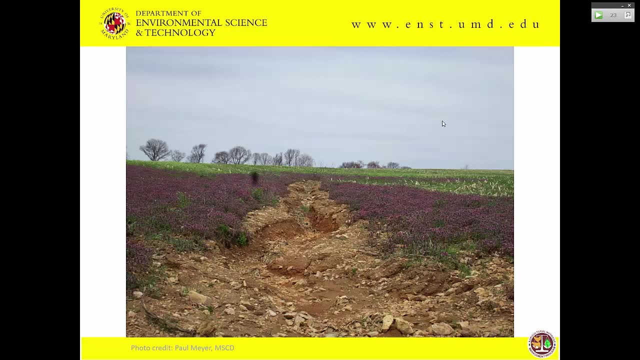 The sand's too heavy and the clay just holds to itself. Same with water, though, You'll often see more silts moving Again the fine textured soils. they don't erode nearly as much, So if you ever see one of these ditches, that can kind of get eroded away. 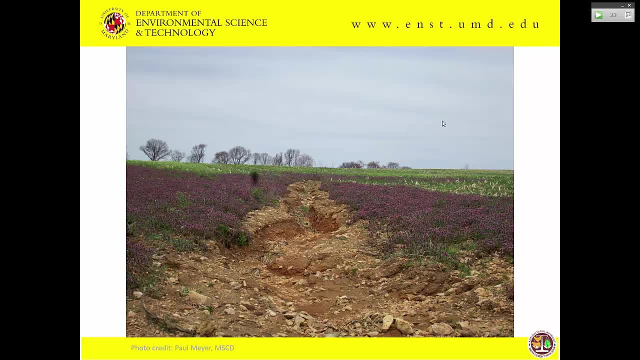 you'll notice always the big boulders, kind of at the top. Again they're just too heavy to move, But at the bottom you'll see these finer soils that have kind of settled out, usually where the water slows down again. 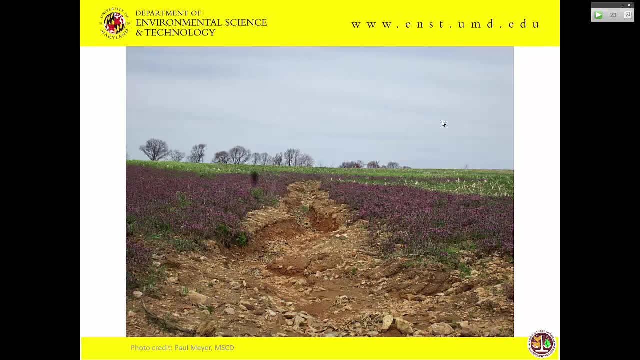 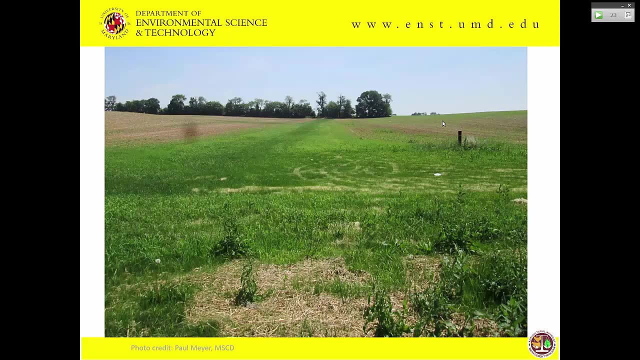 Again, it's just because those silts tend to erode more easily than the bigger heavy things. If you had a grass waterway, you don't have to worry about these problems as much. right? The living roots help hold the soil down, so you don't get nearly as much of this. 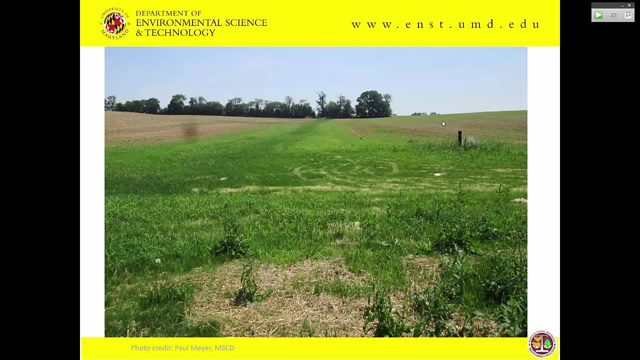 So again, that's kind of one of those site-specific things you want to think about. If you have an area where water tends to flow in a field, you probably want to maybe put in a grass waterway there. It helps reduce erosion and helps keep the big divots out. 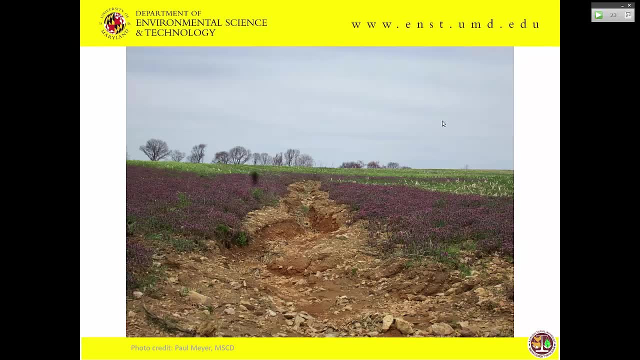 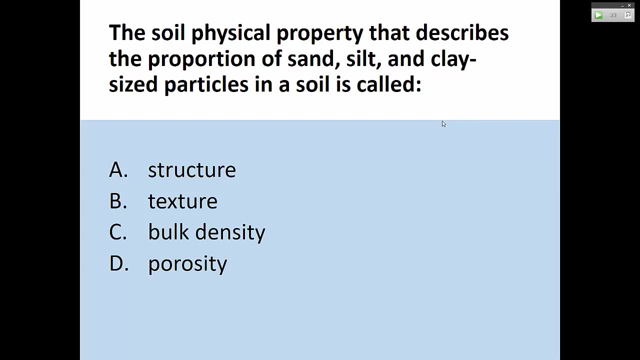 Can you imagine trying to pull a tractor through that? It's not pleasant. All right, so review. What is the soil physical property that describes a percent sand, silt and clay. All right, most people said texture. Yes, Structure is actually something different. 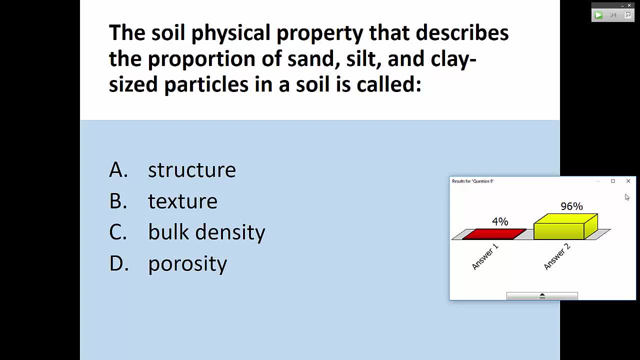 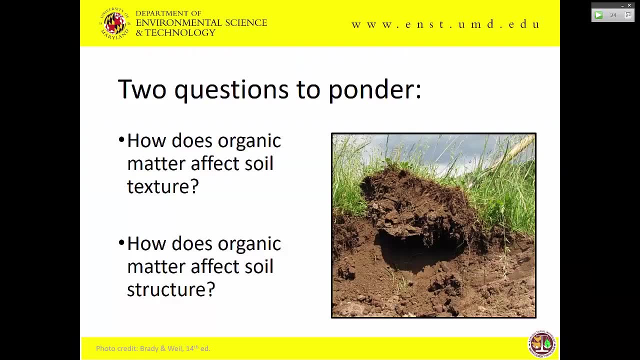 That's kind of how the soil is in, like aggregates and kind of suctions to itself, But texture is sand, silt and clay, So keep that in mind. So next thing: you consider organic matter. How does that affect the structure? 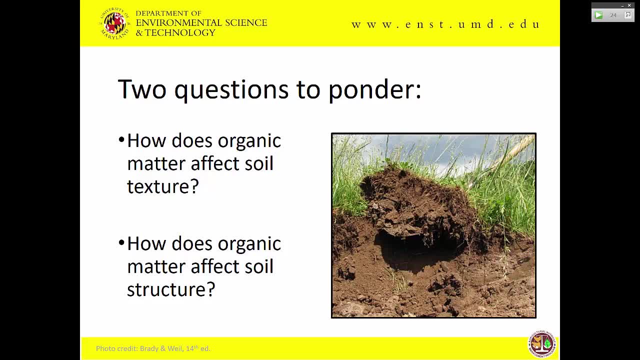 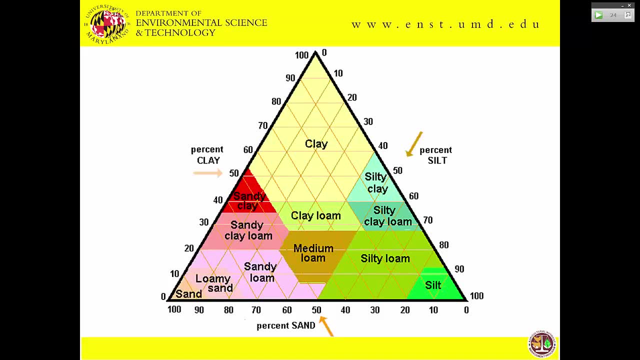 That's our first question to think about. How does organic matter affect the texture? We'll get to the structure later. Look up here. What do you see? Any organic matter up there? Nope, Remember, texture is the sand, silt and clay. 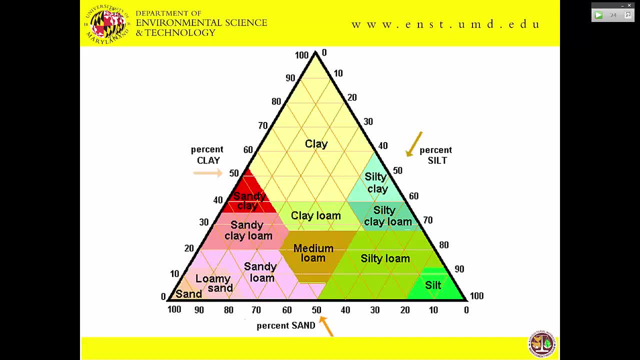 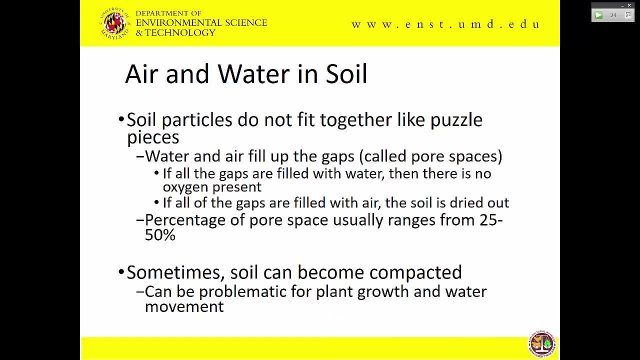 Organic matter is nowhere in that definition. The organic matter has nothing to do with the texture, All right, so that deals with the mineral particles Next up the pore space, so the air and the water. So remember, soil does not fill an area like a puzzle piece, right? 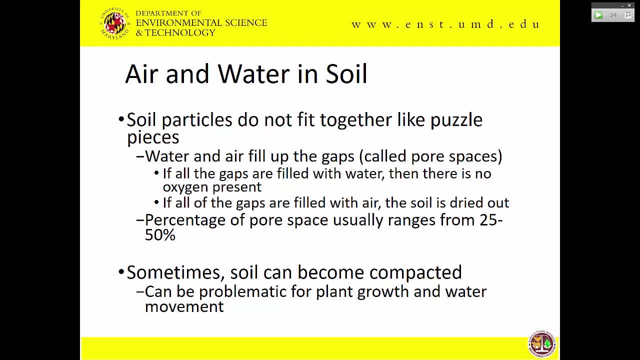 It doesn't perfectly fit together, so there's no gap. I always like to think of it as like: if you put a like, had a beaker put a bunch of marbles in it, would you be able to pour some water still in that beaker? 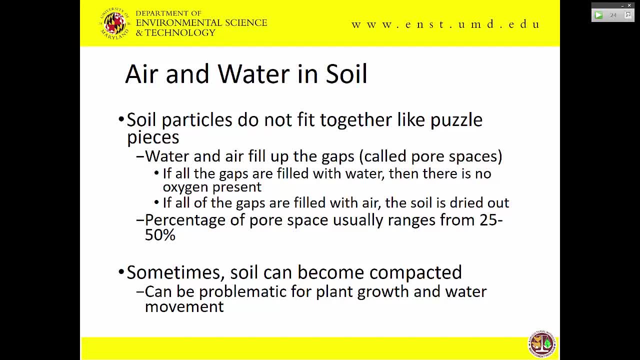 Yeah right, There's space in it, and that's what the soil particles are doing too. You can't see it because it's very small, but there are these pore spaces, So water and air have to fill these gaps. 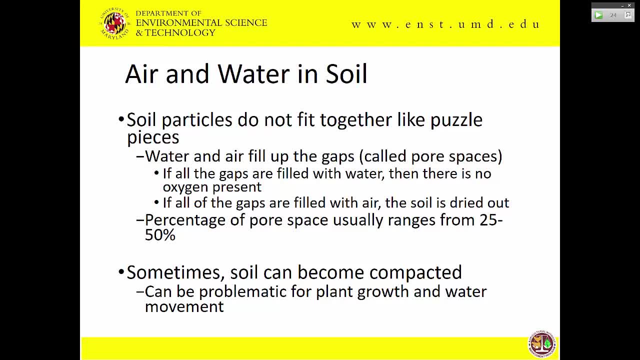 If the gaps are all filled with water, just so it's completely saturated. that's actually bad news because, remember, you've got roots down in there and roots, believe it or not, can actually drown. So if they're in the pore spaces and they don't have any air, they can actually drown. 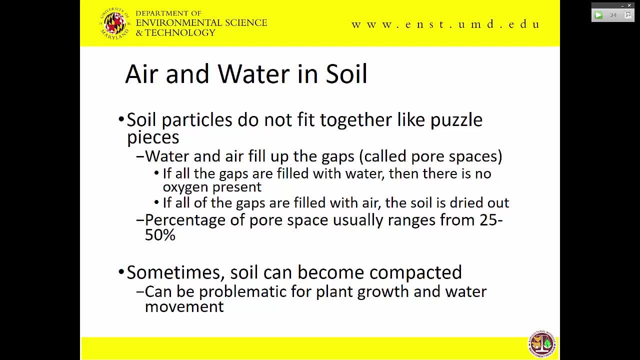 so that's not good news. If the gaps are all filled with air, that's also bad news. so it's completely dried out. you're not getting water to the roots, So you want a nice mixture in there Now- a good soil. a percentage of the pore space will be closer to the 50% range. more. 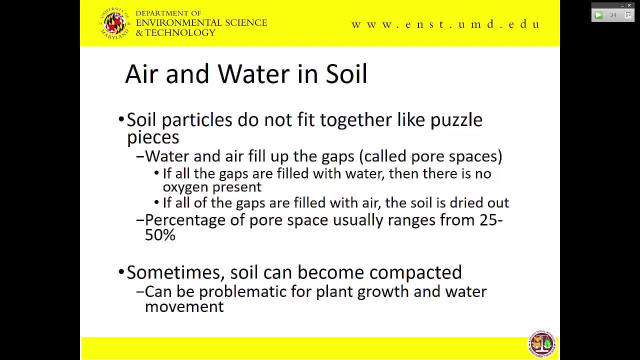 compacted it can get down to 25%, but it depends. Do you have compaction? What kind of soil types do you have? How do you determine how much pore space you have? Now, the soil compaction is a problem. 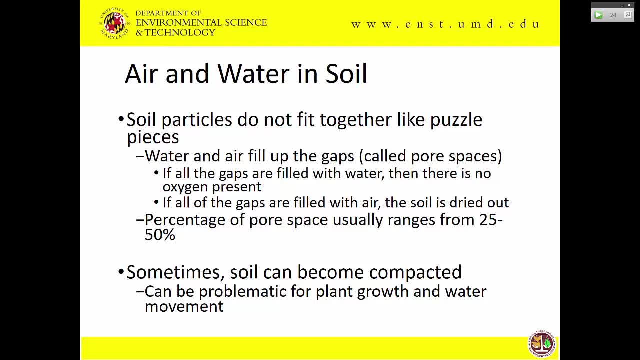 What it does is, if you think about those marbles, all those little holes are slowly connected in some way. They're almost like little tubes going through the soil. But if you get compaction you're cutting off all those tubes and you're ramming all. 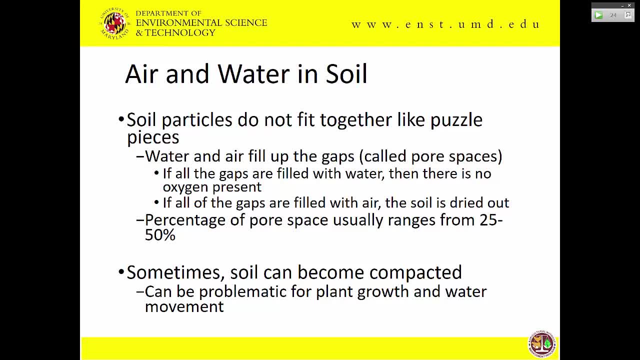 the minerals together. So if you can't get roots down and through there and you can't get water down and through there, that can impact plant growth, In fact a lot of times. I don't know if anyone's ever done this. have you ever had a plow pan? 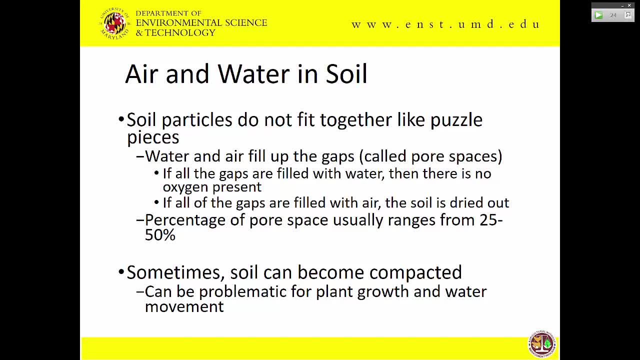 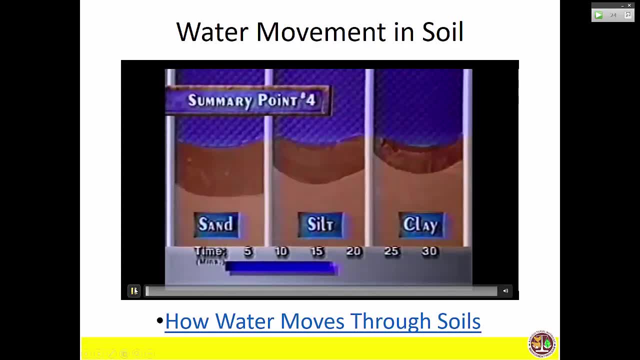 and you dig it up and you see the roots just spread out right at the plow pan. It won't even go into it. Compaction can be a problem. So I do have a little video. Summary point number four: Sandy soils contain larger pores than clay soils but do not contain as much total pore. 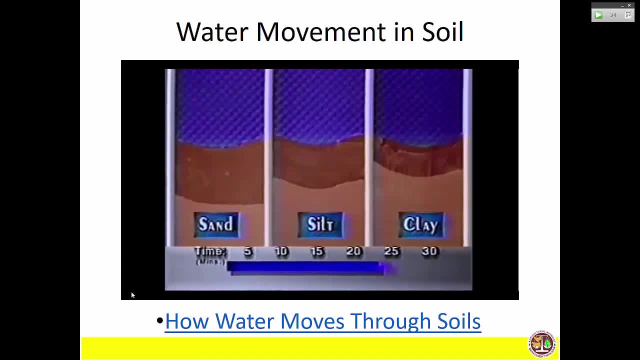 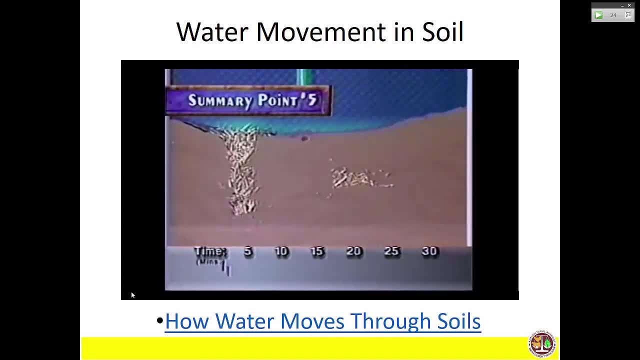 space as clay soils. Sandy soils do not retain as much water per unit volume of soil as clay soils. Summary point number five. Factors that affect water movement through soil include soil texture, structure, organic matter and bulk density. Any condition that affects soil pore size and shape will influence water movement. 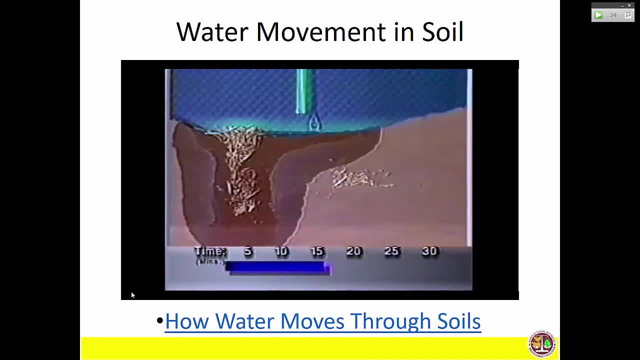 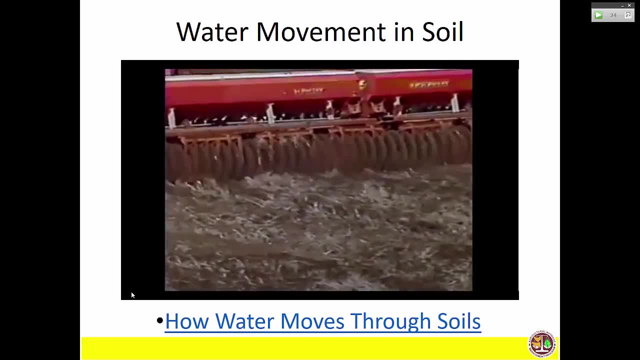 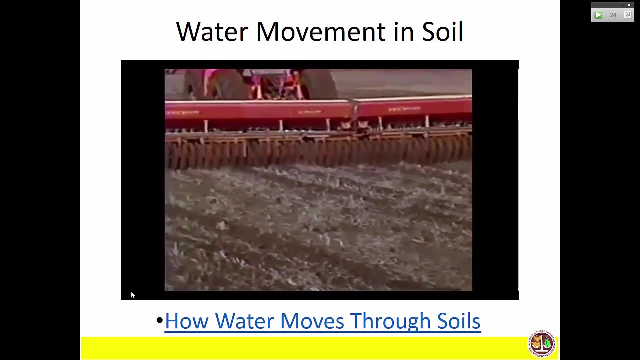 Examples include tillage, compaction, residue, decay, root channels and wormholes, For example. minimum tillage maintains organic matter near the soil surface. When organic matter is used to keep soil pores open to the surface, downward water movement can be greatly enhanced. 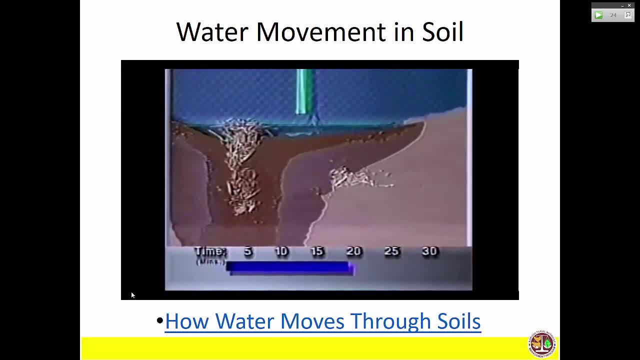 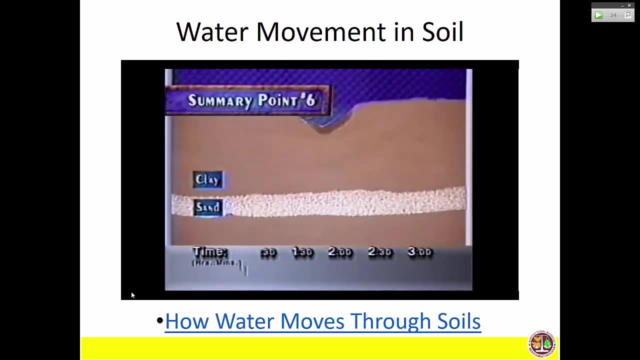 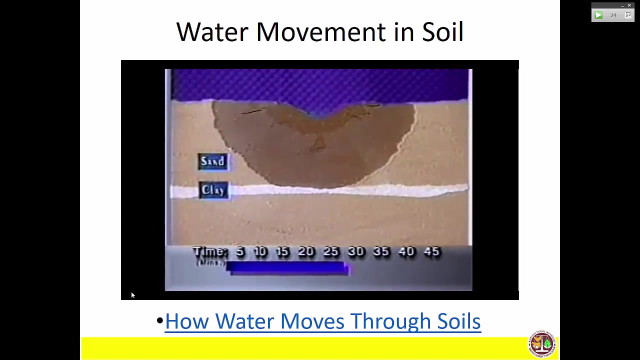 The right side of this model shows organic matter buried under the surface of the soil. Under these conditions, the organic matter restricts the downward flow of water. Summary point number six: Water movement is slower in clay soil than in sand. So when a coarse textured soil, such as sand, overlies clay, the downward rate of water movement 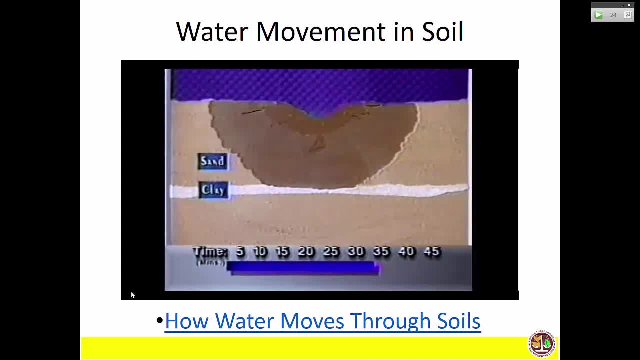 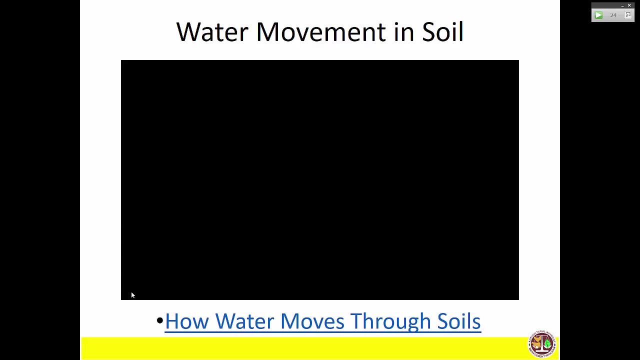 slows once the wetting front contacts the clay soil. This can result in a long-term buildup of a perched water table above the sand-clay interface If water continues to infiltrate the soil surface. So I thought that was kind of interesting, because it not only shows you how the water 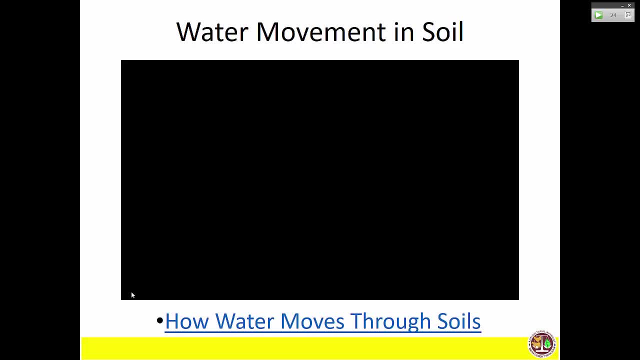 moves through the soil, different textures. right, It's faster than clay. But think about that first diagram. It had sand. It showed you it moved faster. And then it had clay. It was like half as fast, right, But they added the same amount of water to all three of those. 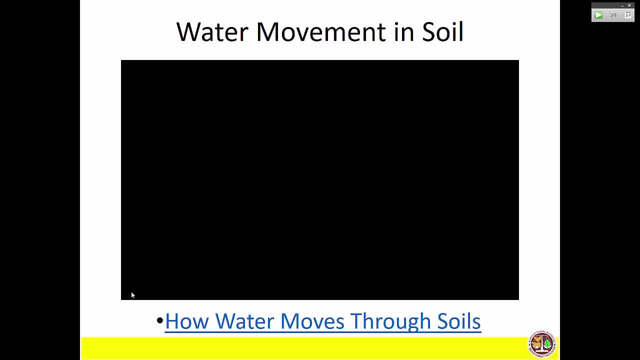 So what does that mean? Does clay hold more or less water? More right, It held the same amount of water in much less volume. So it means pore space in the smaller or the finer textured soils is going to be higher. 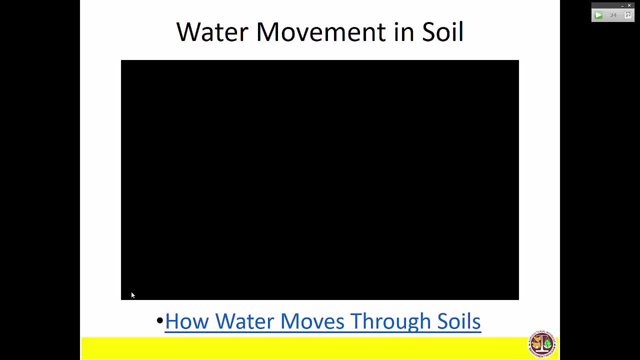 Even though it's smaller, so therefore things move slower. you're going to have a lot more pore space in these finer textured soils. The other thing that I thought was cool was how it showed the tillage. If you have roots and things that are on the surface, they can actually help infiltration. 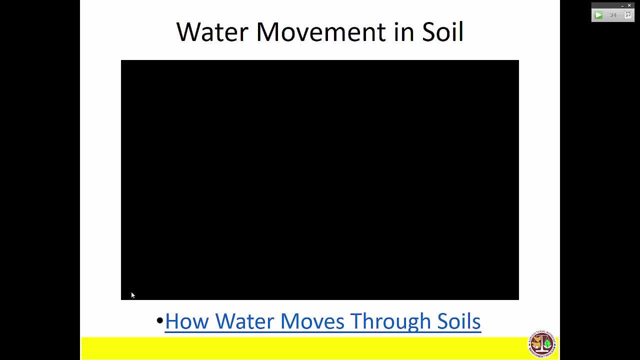 increase versus if they have a lot of stuff buried and it's not connected to the soil. that actually seemed to impact the soil. It just seemed to impact, like it kept the water from flowing into the soil as much. So I thought, oh, that's kind of interesting. 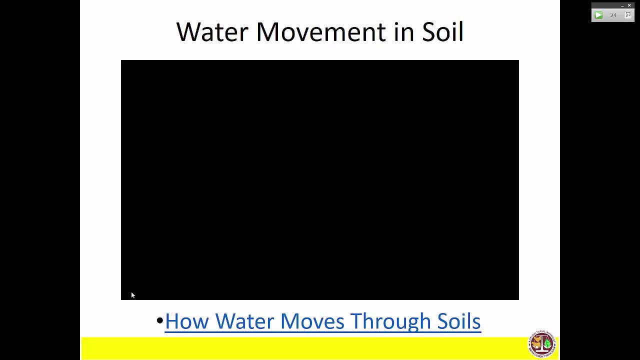 You have to think about the benefits of conservation till versus moldboard plowing, how that kind of increases infiltration, decreases runoff. But then if you have a lot of nitrate in your soil that can also increase groundwater pollution. So you kind of have to think about all these tradeoffs. 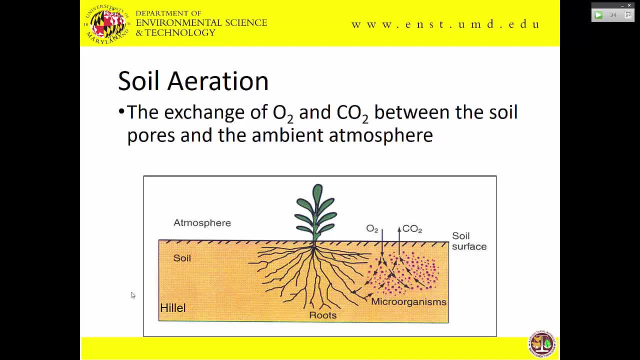 So water is important for how it moves with nutrients, right, But you have to think about air too. Like I said, plant roots: they do not photosynthesize, do they? They're underground, They don't have access to the sun. 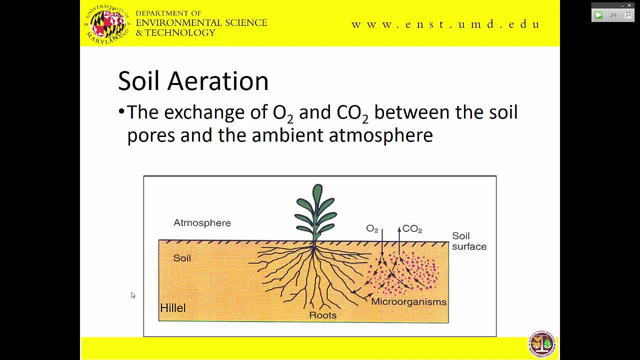 But they're still cells, which means they have to respire. So they need access to oxygen, just like you and I do. So if there's pore space in there that has air in it, they're getting oxygen. But if you've got water in there filling up all the pore spaces, they don't have access. 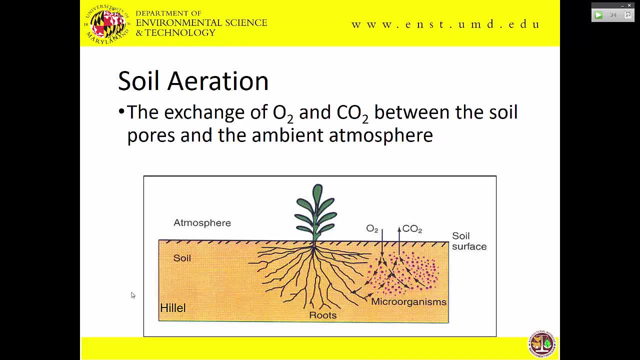 to the oxygen that they can use. They can't use the oxygen in the water, So therefore they can actually drown, And you can kind of see that In really bad years where you have clays and things like that, not only will there. 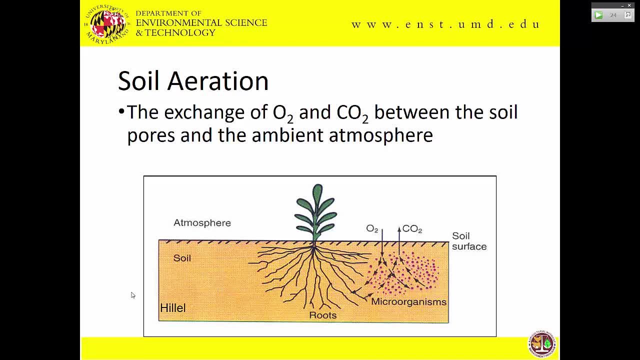 be nutrient issues, but you can actually drown your plant roots out too, So they need access to air just as much as they need access to water. Now, believe it or not, we actually have. well, I mean, you should believe it. 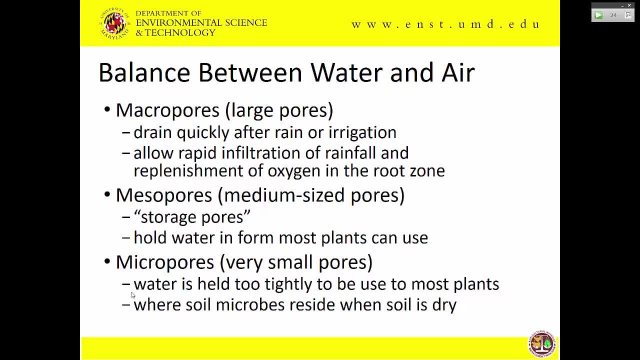 Scientists are crazy and we classify everything, But we have different names for the different pore sizes. Macropores are the really large things. I like to think of these as the wormholes, right, The kind of big holes in the soil that you can see. 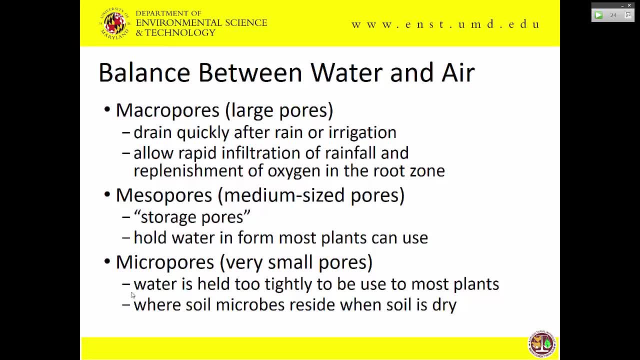 They drain quickly, obviously After rain or irrigation, So they can be useful And they help with infiltration, But sometimes these are the ones that drain first, So they're not necessarily going to help plants. The mesopores: these are the medium-sized pores. 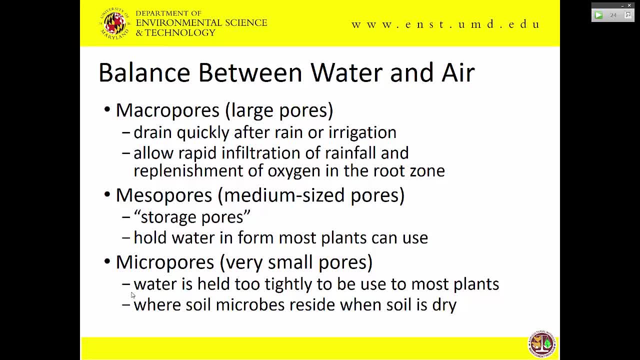 These are what we consider the storage pores. This is where the available water is for plants. These micropores, these are the ones where it's so small that the water is held so tightly against the soil particles that the roots can't access it. 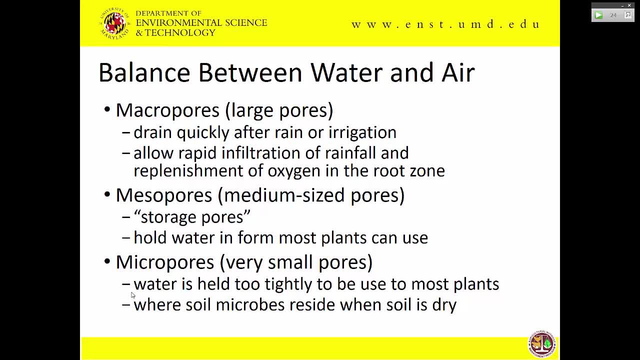 It's there, but they can't pull it away from the clay. So you want a little bit of all of these, because in the tiny ones that's where soil organisms can go, like the bacteria, et cetera, when it's really dry. 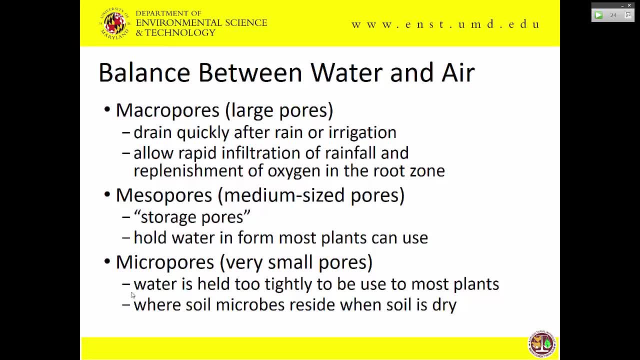 But you do want the mesopores to have some water too, because that's where the plants can actually get it. Has anyone ever had a sponge At some point? you can keep squeezing it, but you can't get any more water out. but 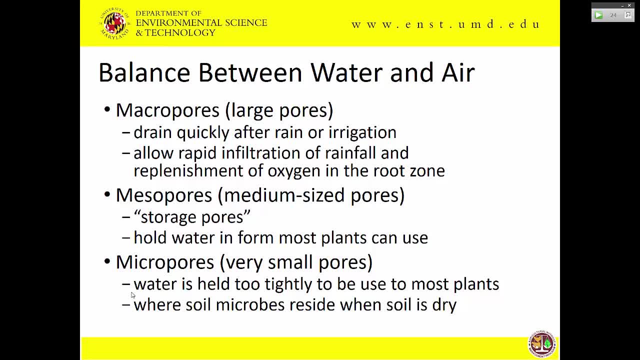 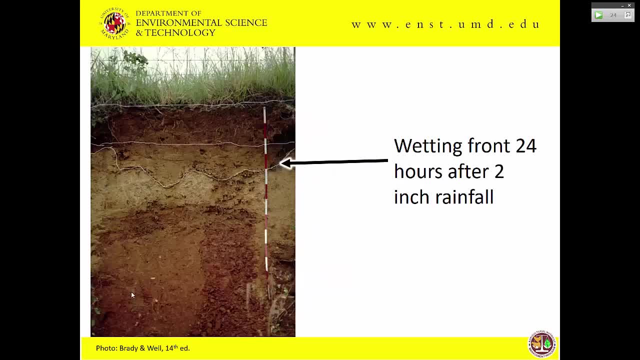 you know it's not dry. It's kind of what we're thinking about here. At some point it gets to the point where there's still water there, but you just can't get it out anymore. So here this actually shows it had been dry for a while and then it rained and they 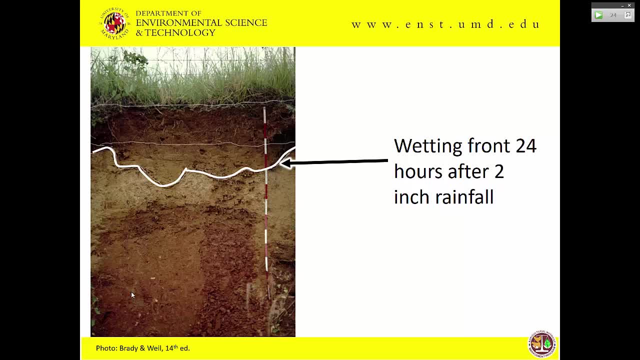 got nice two-inch rainfall. You can actually see kind of along that white line, the wetting front. See where the color changes there a little bit. Why do you think it's wavy like that? Why would it be wavy? 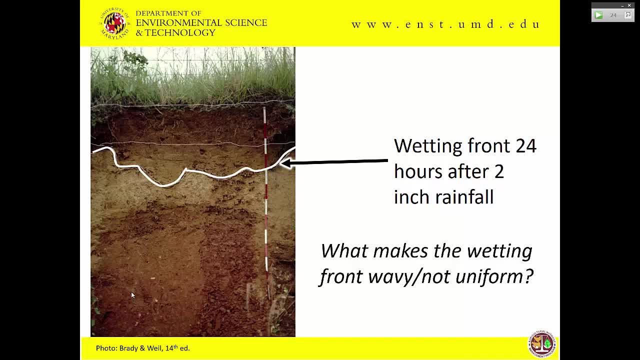 Depth of plant roots. A little bit of depth of plant roots will help infiltration a little bit. Anything else possibly? I know we don't have all the details, but ideas Could be like organic matter in here. Yeah, Could be organic matter. 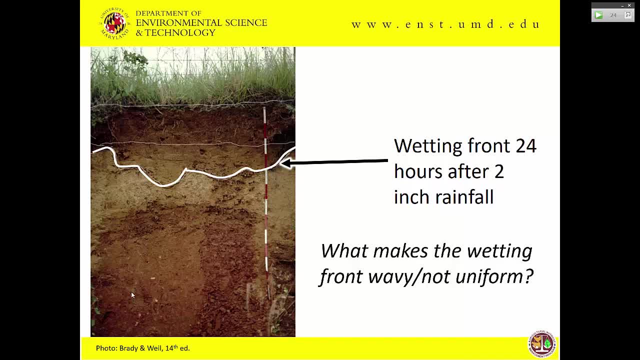 Organic matter acts like a sponge too. It can hold some water and get different amounts. What else? What's the other thing that impacts how fast water moves? The soil texture- right Soil texture- Yep, You could have a little bit like. even a couple inches away you could have soil textures. 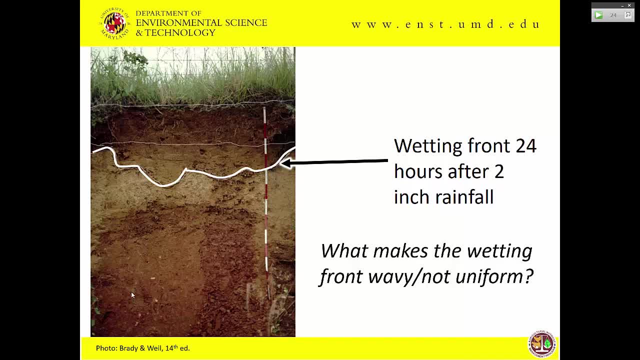 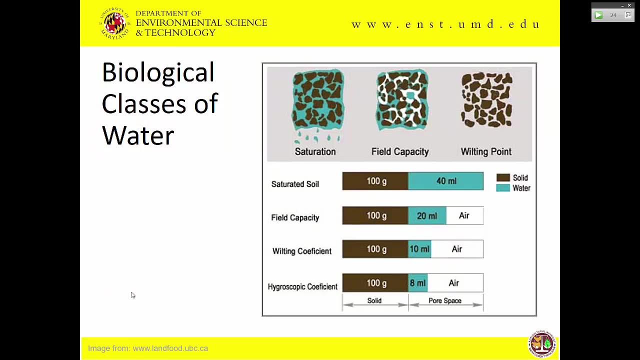 changing enough that it makes the wavy uniform front. So organic matter, soil texture, all of these things impact how water can move through the soil. Yeah, Okay, Now again, we like to classify things, so we classify how much water is in the soil. 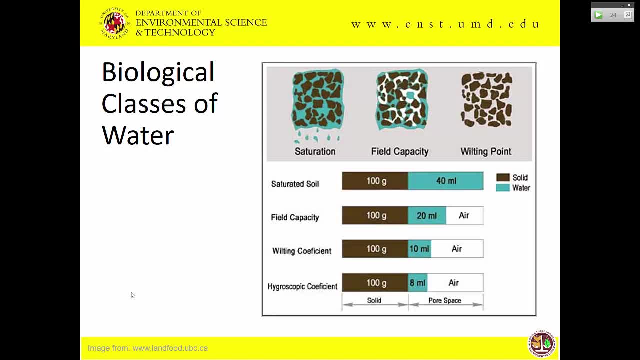 So obviously I've talked about this before- All pore space is filled with saturation. That's after a good day long of two inches of rainfall, Not the really fast splashy kind, but the kind that just kind of just came slowly over. 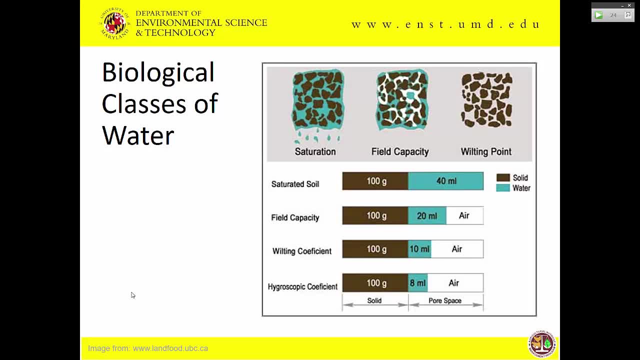 one or two days. That's when you get saturation, And plants can tolerate this for 24, 48 hours, But it's when it's longer than that, Yeah, When it's longer than that- that's when they start getting into trouble. 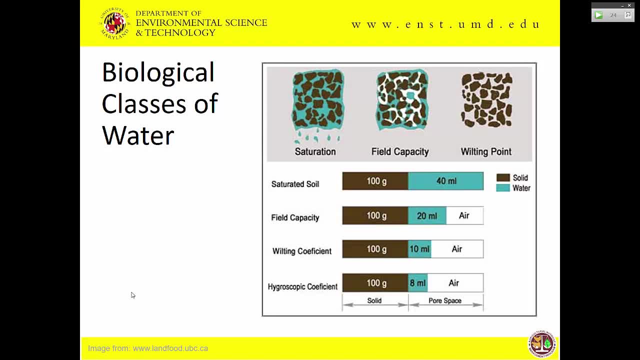 Now, after about 24 hours, all of the water will flow out of the large, those macro pores. We call that free gravity water, because it's the stuff that's going to move the quickest And we get what we call field capacity. 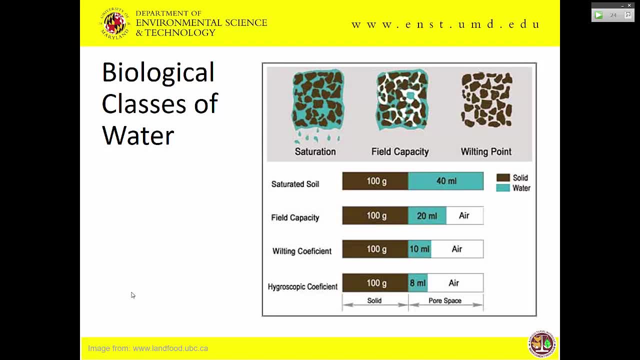 This is about how much water the soil can hold when it's not saturated. Now the wilting point: that's when the water is. There's still water in the soil, but the plants can't get it anymore, So that's when you actually start seeing wilting. 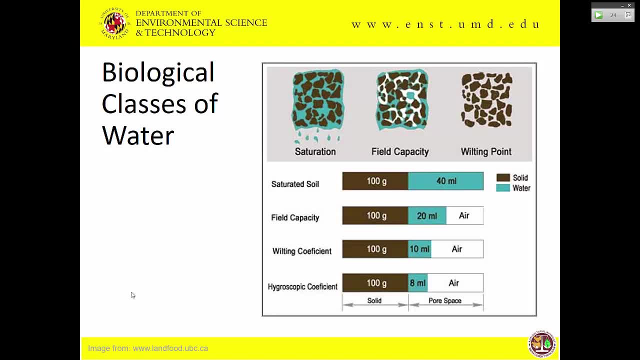 I just planted a couple of plants this past summer and then we just got this dry spell and I wasn't paying attention to watering. They were wilting pretty badly. Plants can wilt and they can rebound if they get water pretty quickly. but there gets a. 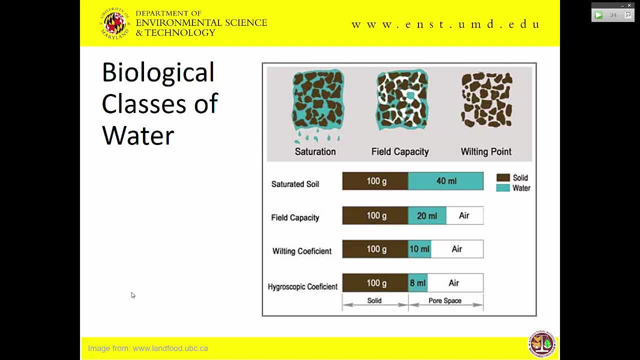 point where they can't rebound anymore. So those are kind of the things to know: Saturation, field, capacity and wilting point. And obviously, because we have different soil textures, it's going to be different for the soil textures too, right? 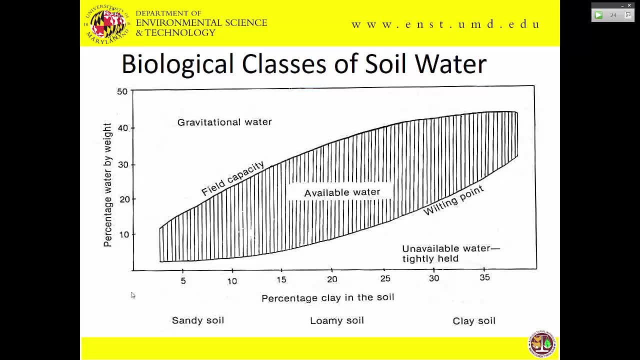 So here we have percentage of clay in the soil, so sandy soils versus clay soils, And then you have the percent water by weight. So what you should notice is that this line is field capacity. It increases as you go towards the clays right. 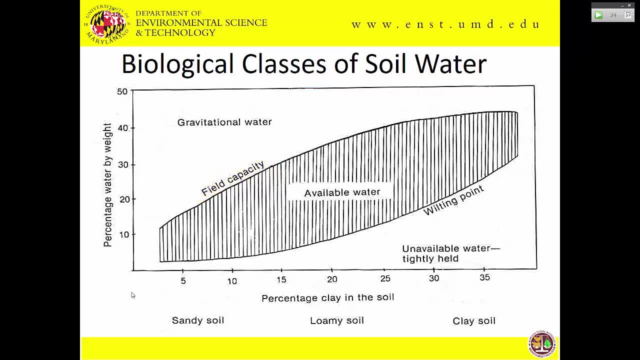 So, like we talked about, clays can hold more water in their field capacity. And what's field capacity? again, Field capacity is usually about how much water is in the soil after a soaking Rain event, like 24 hours after that. 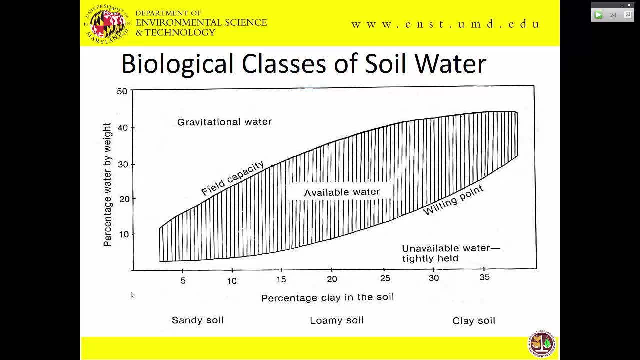 So it's kind of the amount of water it can hold that's not flowing by gravity, Notice. the other thing that increases is the wilting point. Remember clays. they not only hold more water, but they have smaller pore space too. 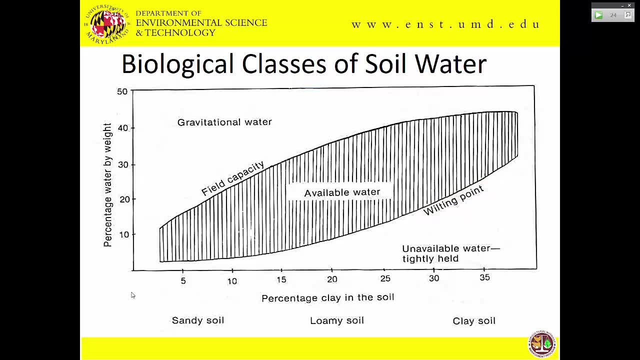 And those tiny pore spaces, those micropores that hold the water so tight that plants can't get to it, which means there's going to be a much higher wilting point. So it can hold more water, but it gives the plants less access to said water too. 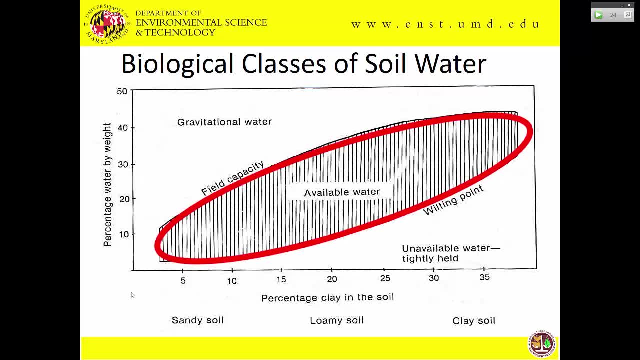 Does that make sense? So the available water is kind of in between them. At field capacity, that's when you have the very most available water from the plants. At wilting capacity: right above that is where you have the very least amount. 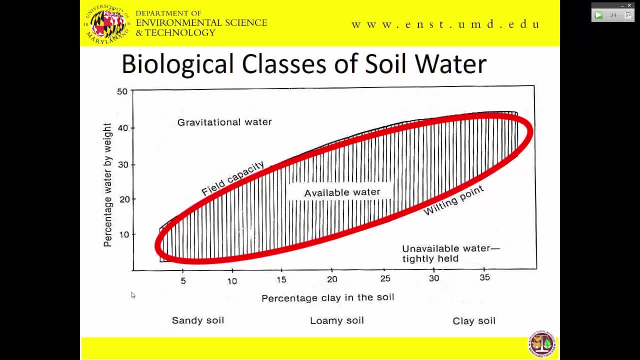 At wilting point, they're having a real hard time surviving. So, above field capacity, that's what we call the gravitational water. That's water that isn't really bound to the soil, It's not being held back by it, It's just flowing down due to gravity. 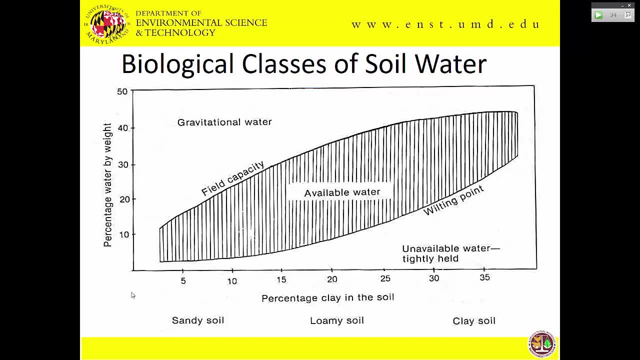 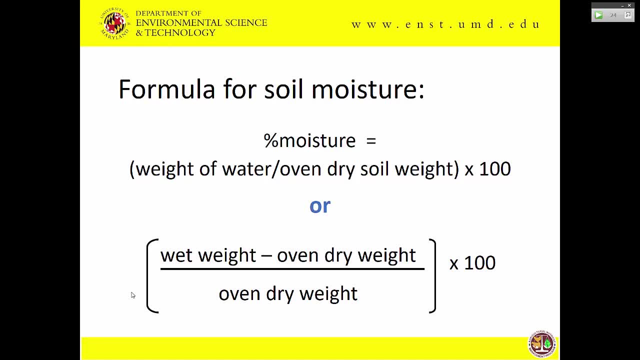 Below that it's obviously unavailable. So while we're talking about it, let's do the formula for soil moisture. Soil moisture is something you could be expected to calculate in the exam. Yes, they will have calculations for you to do. 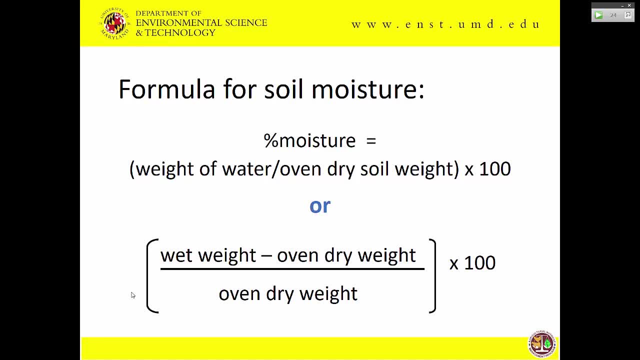 I know you don't get a notepad to bring for formulas so you want to memorize these. I think they will let you have calculators that they supply. I think I'm not sure We do. You can use a calculator. 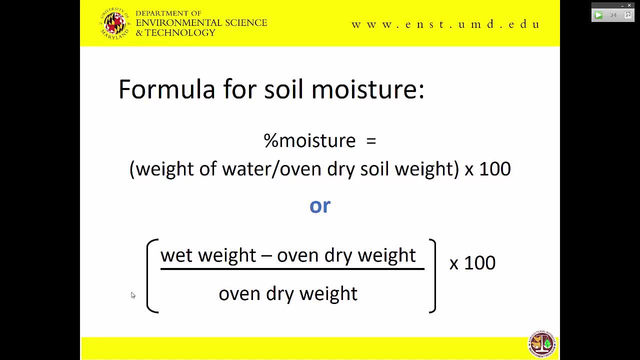 You just can't use a phone. Yeah, Oh, okay, All right. So percent moisture in a soil is going to be the weight of the water divided by the oven-dry soil weight. So it's how much water is in there divided by the soil weight times 100.. 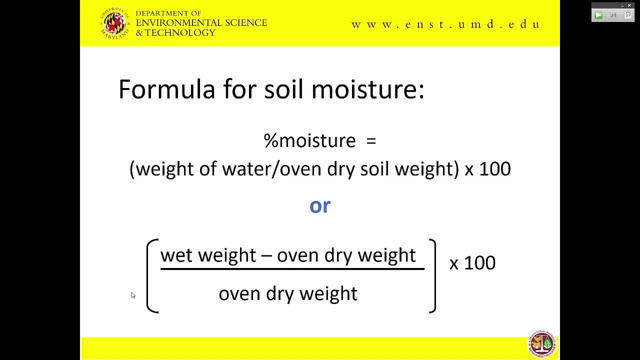 So you may ask yourself: how do I find out the weight of the water? That one's pretty easy: You take the wet weight of the soil, dry it out in an oven, subtract the two and that's how much water was lost. 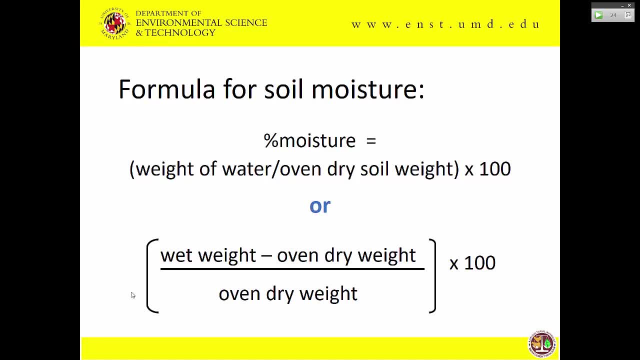 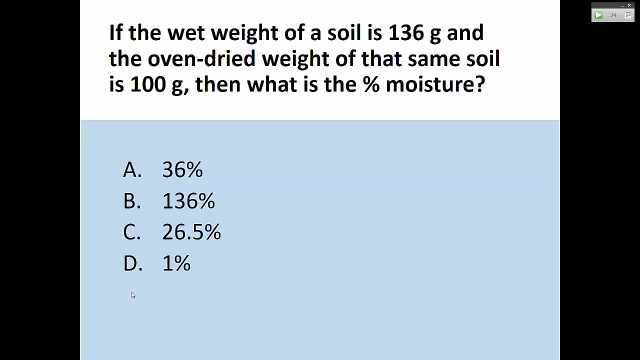 Divide that by the oven-dry weight, multiply it by 100, and that will give you the percent moisture You good. You ready to practice this one All right. Wet weight of the soil: 136 grams. Oven-dried weight is 100.. 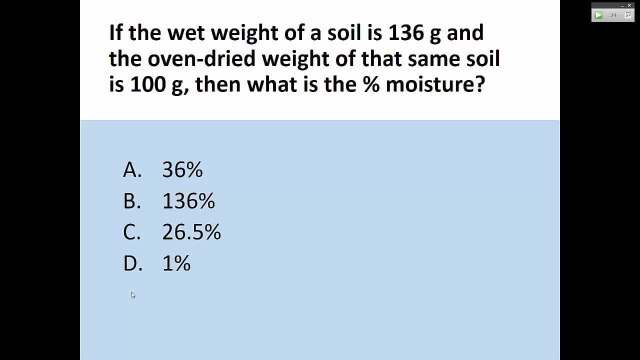 So what is the wet weight of the soil? 136 grams. So what is the percent moisture? All right, Let's see what you said. Most people said 36%. Let's check it out. So 136 minus 100 is 36 grams, right? 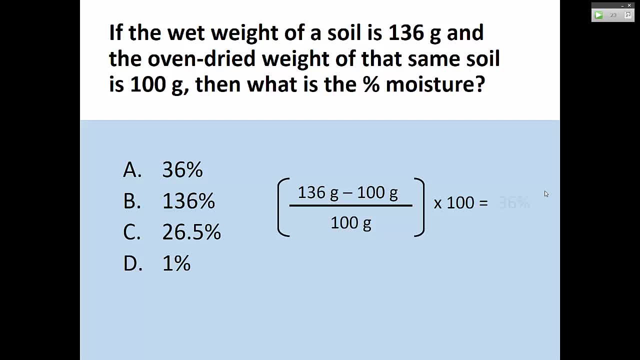 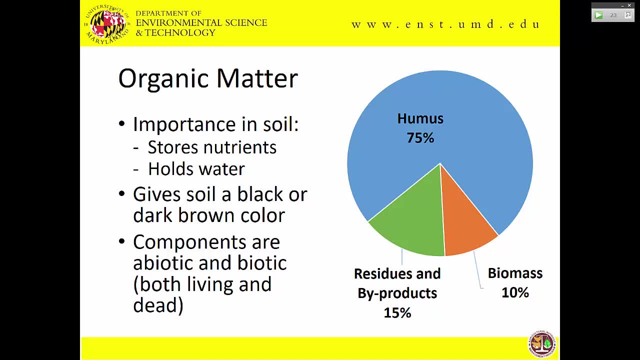 36 over 100 times 100 is 36%. So what's he got All right? Next up is the organic matter. I sometimes refer to this as OM Just because I'm lazy. So just so you know what I'm talking about if I say the OM. 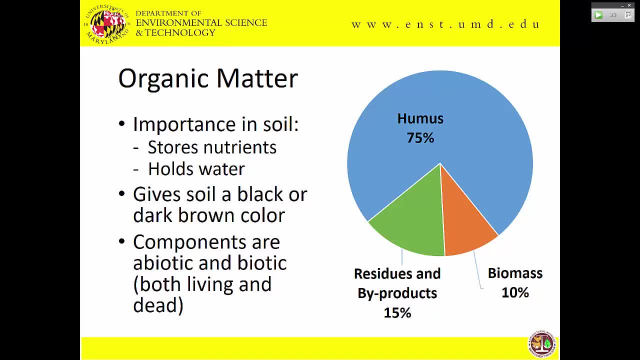 Now this is important. in soil It's kind of like the clay: It holds on to the moisture. So having organic matter can store cold water and also storing nutrients for you. It's similar to clay in that regards Clay likes to hold on to things, so does the organic matter. 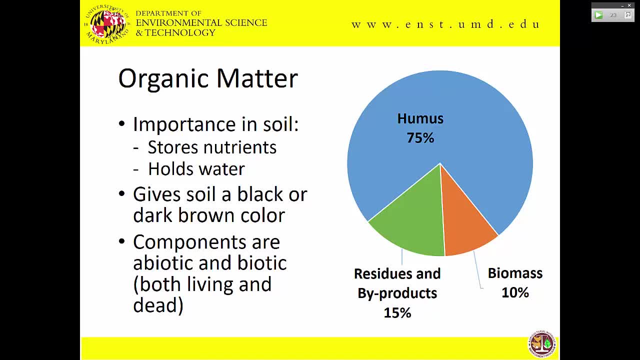 Now this is actually what gives soil a nice black or brown color. You ever see topsoil being sold in the stores. What color is that? Hmm, It's black Black. Yeah, That's because it has a lot of organic matter in it. 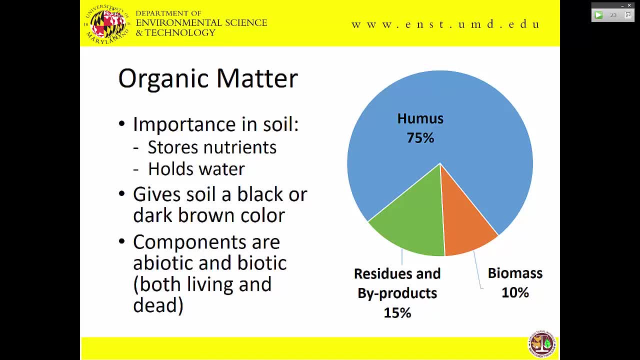 Unfortunately, my house was built in the 70s and they stripped the topsoil off, built my house and then didn't put any topsoil back on, So I'm having yard issues. I just bought it recently, so I'm working on those. 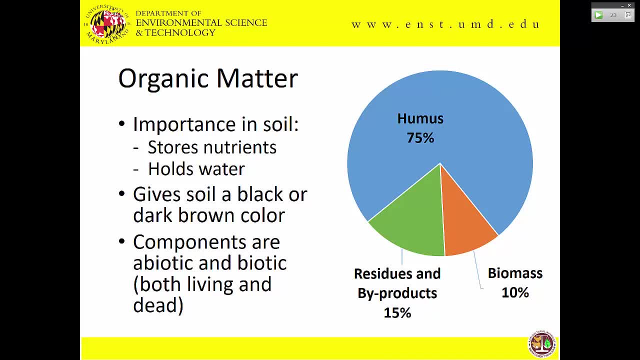 Soil scientist with a bad yard doesn't look good. So the things to think about are that these components are abiotic, which means nonliving, as in like chemical and also biotic, and it can be both living and dead. So you got like nonliving, neverliving things, and then living or once-living things. 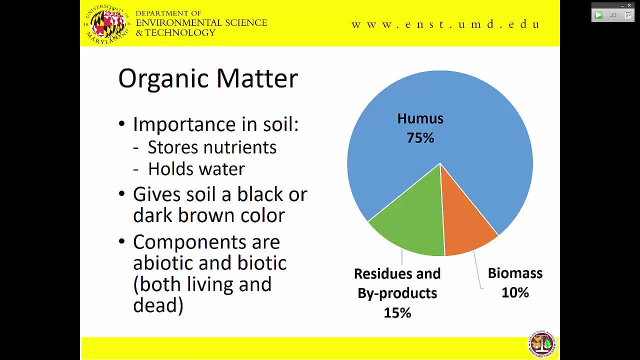 So things like humus is about 75%. That's usually what gives it its dark color. Biomass or the living things make up usually about 10%, and then the kind of crazy residues and byproducts that these things make, even while they're decomposing, makes up another. 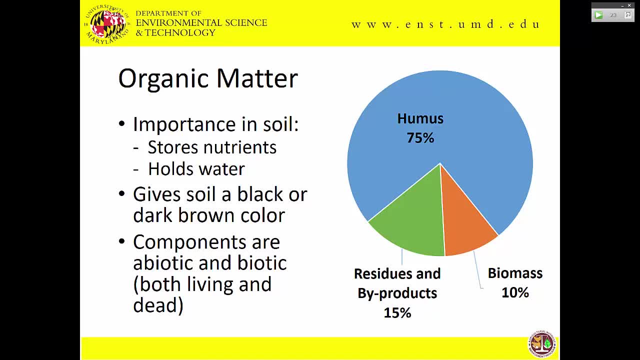 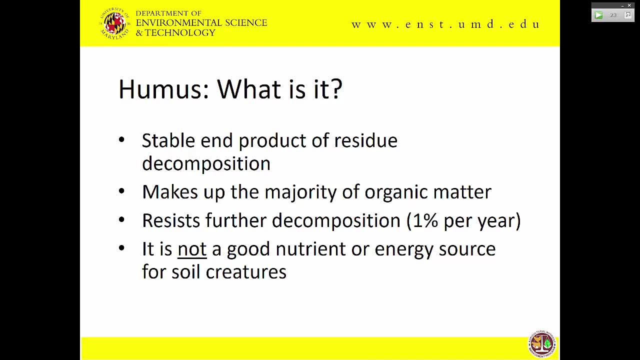 15%, But it's mostly this humus. Now, the humus what it actually is is. you know how things decompose. The humus is, when it gets to the point where it can't decompose anymore, Like it'll decompose a tiny little bit. 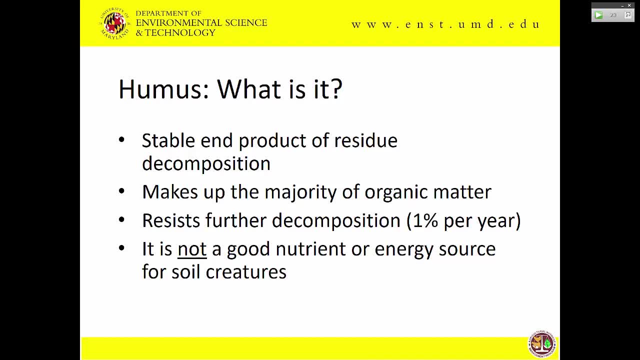 There's a few types of bacteria that can break this stuff down, but it's pretty resistant, So that's essentially what it is. It's when you get to the point where there's not many living things that can get much more energy from it. 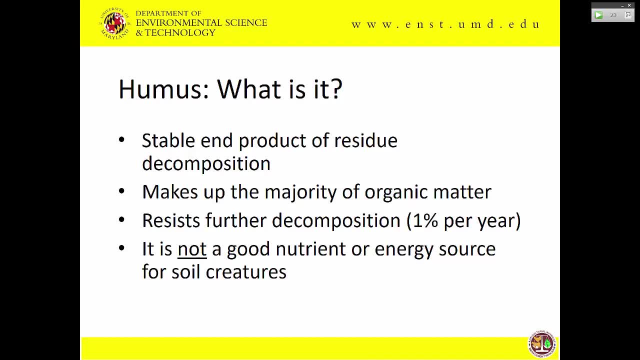 Not a very good nutrient source, though This stuff does not actually have the nutrients. It has the nutrients inside of it. It'll hold onto the nutrients for you, but it doesn't actually provide the nutrients And it's not a good energy source. 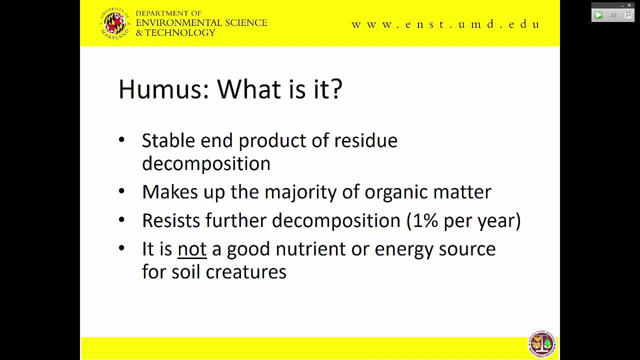 I remember all living things that don't photosynthesize need to eat carbon. That's where we get our energy from breaking up carbon bonds in our food. So this has carbon in it, but there's not a lot of things that can get to that carbon. 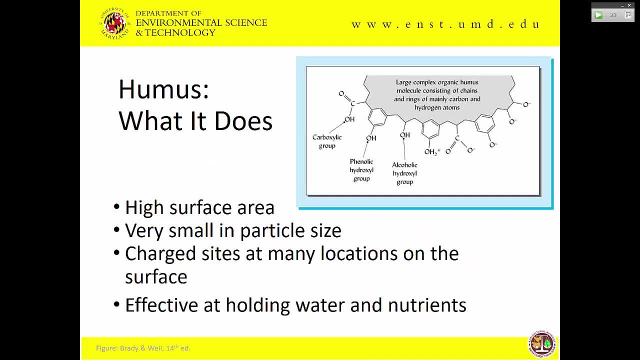 so it's not a very good energy source. Now, like I said, though, it does like to hold onto things. It has a very high surface area, and you've got lots of different places, lots of different chemical structures that'll hold onto things for you. 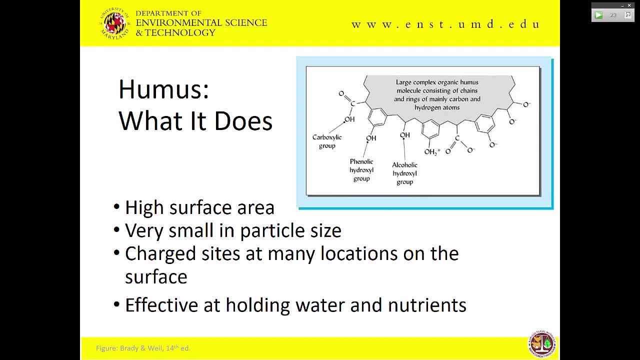 So it can hold onto those things. So that's why we say it's effective at holding water and nutrients. So you want it in your soil. Despite it not being a good energy source or a good nutrient source, it holds onto those. 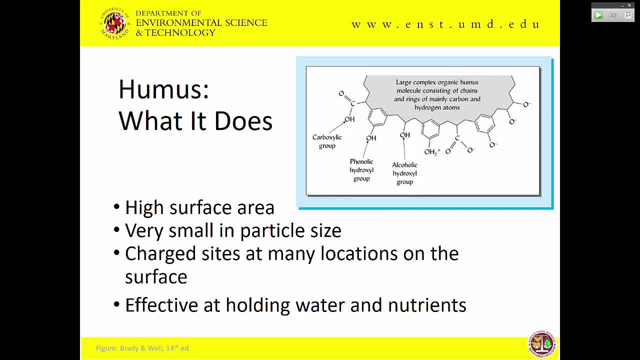 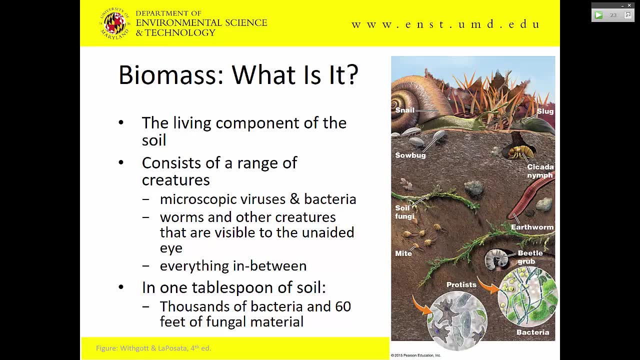 things for you, So you do want a lot of it in your soil, Biomass, the living things- These are the things that do the nutrient cycling. Remember when plants, roots et cetera, die, you've got lots of nutrients in them. but 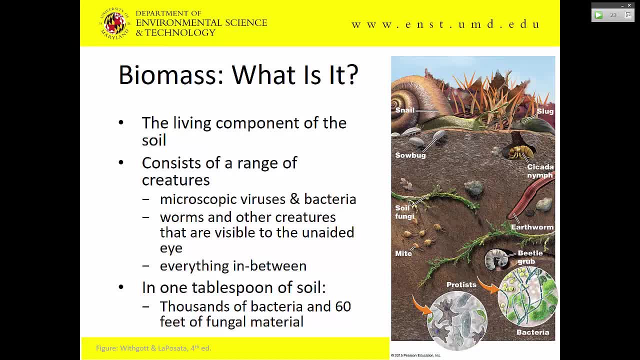 they're not really available to other growing plants. You need to have the bacteria, the protists, the beetles, the worms that help break it down into plant-available forms. So the biomass is actually really important for nutrient cycling And that's why we actually see a lot of emphasis on soil health these days. 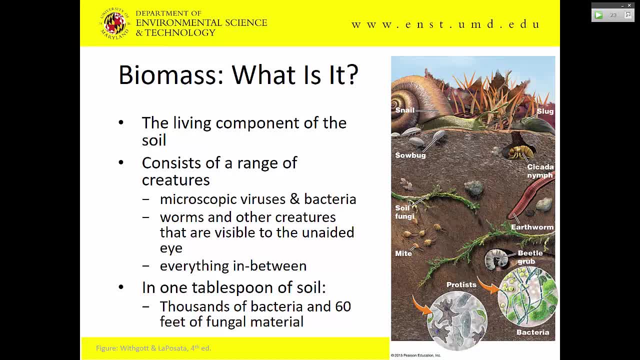 Have you heard that flashy word soil health? That's because for a long time we added a lot of pesticides and things that ended up killing a lot of the living things. So then we've had less nutrients, So a lot of people are finding out that these living things are actually good for the soil. 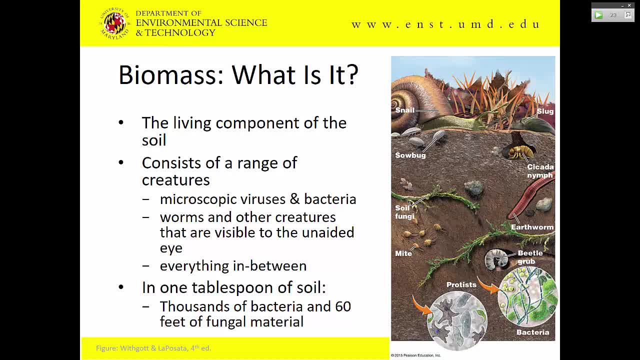 and we want them there. That's why there's more and more emphasis being put based on thinking about your soil health. And it's a whole host of different things, Like I said: bacteria, cicadas. The cicadas even actually do some of the stuff. 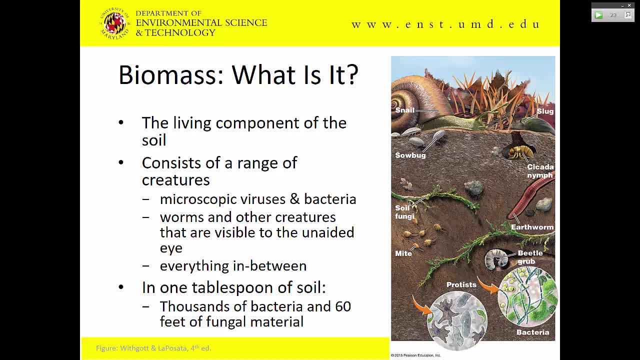 The worms, the snails, They say. in one tablespoon of soil it contains either thousands of bacteria- I've heard some studies say millions of bacteria in one tablespoon And 60 feet of fungal material. Who would have thought? Every time you take a step on the soil you're killing something. 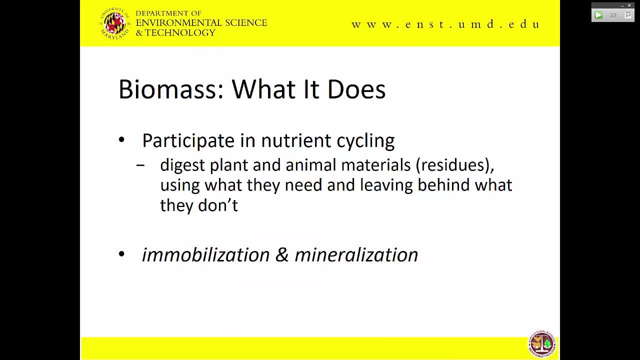 No, I'm just joking. They're more resilient than that. Like I said, good in nutrient cycling. They not only digest things, They make a plant available, They also provide some of those residues that help the soil stick together and provide homes. 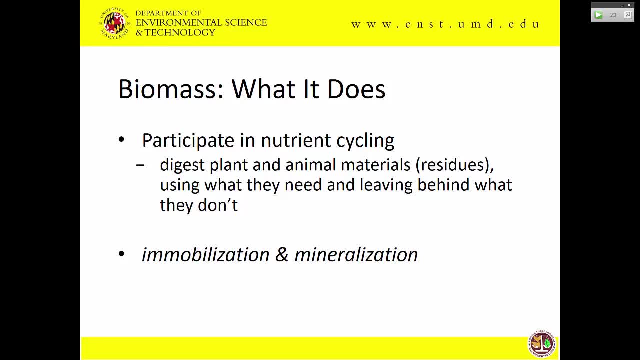 to other things. And don't forget: not only do they help release some of the nutrients, but they do take up some of the nutrients too. You and I all need nitrogen and phosphorus, right? That's one of the reasons why we eat, besides the energy. 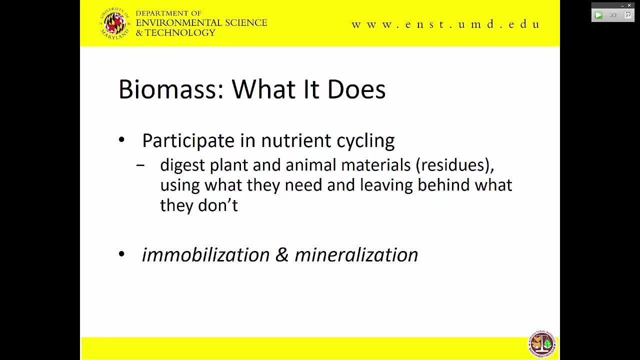 All these organisms eat and get those nutrients too, So while it's in their bodies before they die, that's called immobilization. It's not available to plants, So there is a little bit of this balance going on. The other thing they do is they create those biopores. 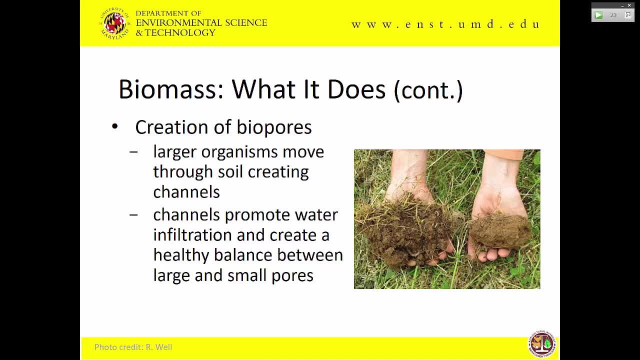 Think of those earthworms coming up, making those big holes. That helps get water into the soil, helps with infiltration And it helps make, because you get the big worms, you get the small worms. it helps make a nice collection of those different pore spaces. 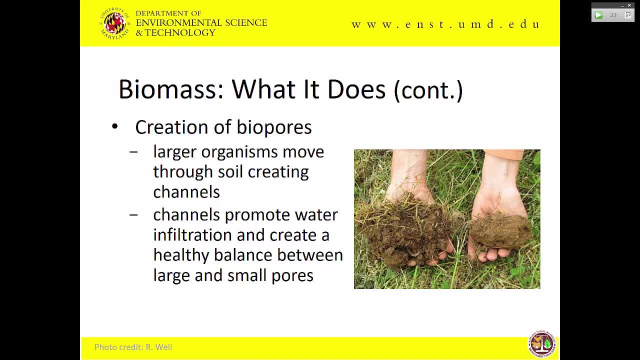 Again, you want a good mix of macropores, micropores and mesopores, because all three of those things do different things and have different services. This plot on the left is from an area where you have a nice worm population. 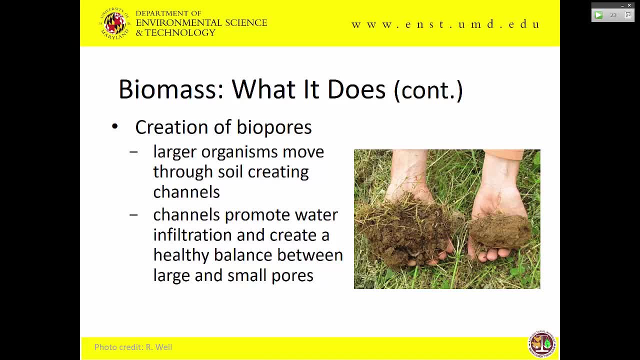 This area on the right not so much, And again you can kind of see, right, This looks a lot more fluffier. You see a little bit of organic matter in it. right, It's a little darker than this other one. 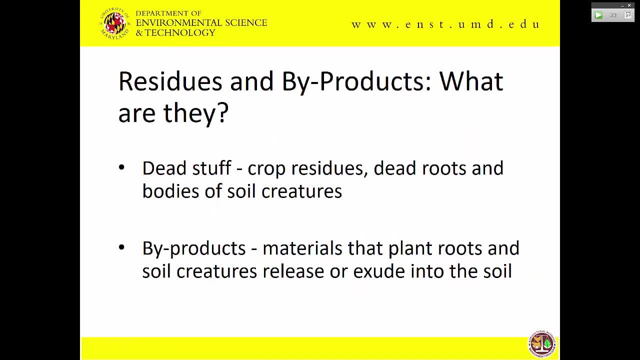 There's lots of different things going on that can improve your soil. So what about the other stuff, The residues and the byproducts? This could be either the dead things, Dead things that were once living, Crop residues, dead roots, et cetera. 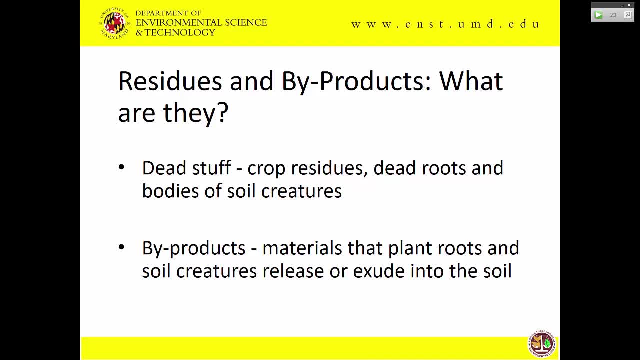 It could also be byproducts. There's a lot of things that roots actually exude or other living things exude to either help with nutrient capture, or I think there's even this one type of tree. It's called a neem tree. What it does is it exudes a toxin. 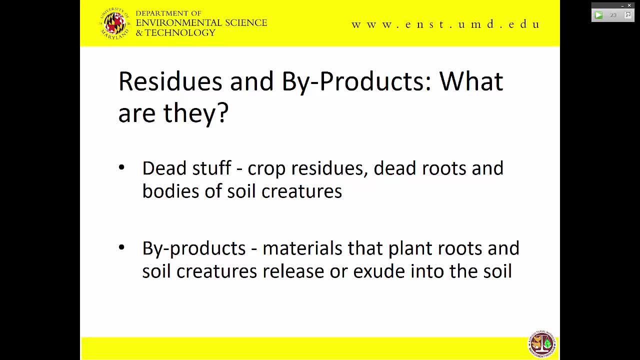 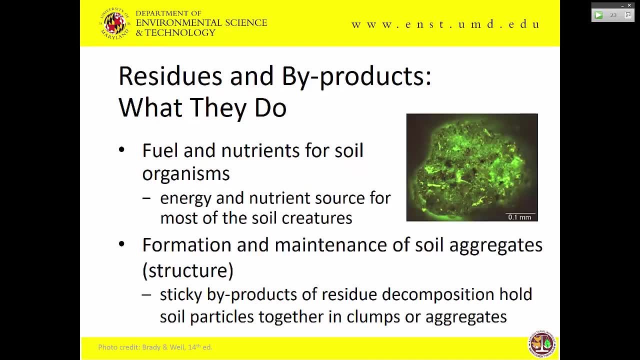 Nothing else but other baby neem trees can grow underneath it. So even like, those kinds of things can be a byproduct that are in the soil. This picture is cool. What they did is they found a way to make one of these types of exudates glow so that 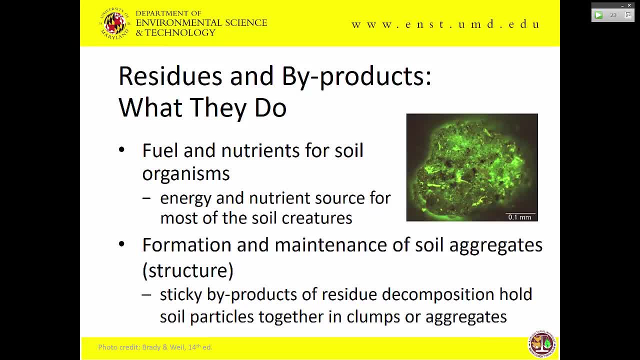 they can study it. So this is one of those byproducts glowing in a soil and you can see how full of it it is. So that's all the stuff that helps. It's literally the glue of the soil. Now, what they do? they provide fuel and nutrients. 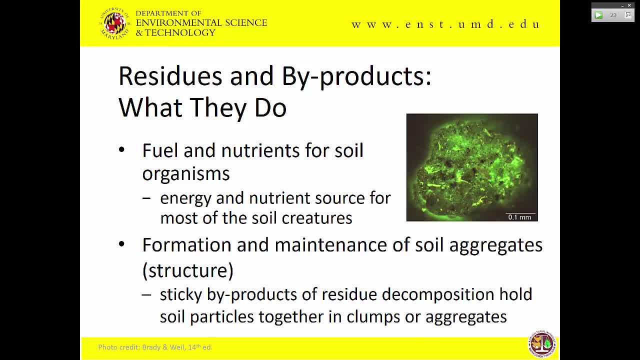 Again, dead things need to be broken down. They provide the carbon, And most of the soil creatures are kind of feeding on this stuff. But the other important thing is the glue. Soil aggregates are what's considered the structure. These hold the soil particles together in clumps. 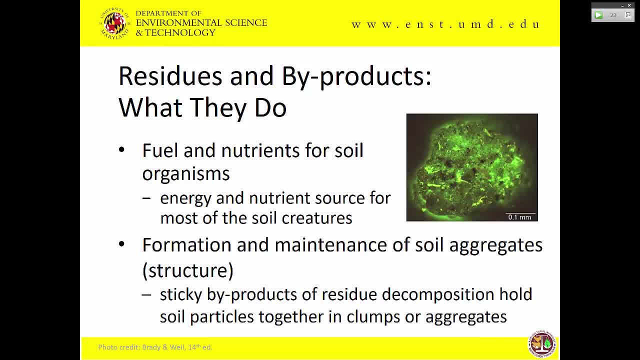 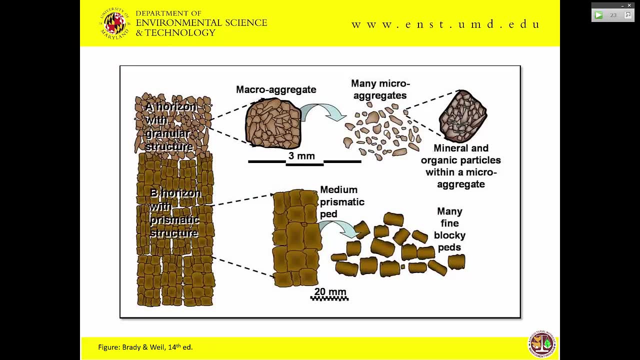 And this helps with infiltration. It helps with your soil health, getting lots of little things to live there, etc. So soil aggregation or soil structure is also really important And you can see lots of different soil structures Depends on what soil type you have to begin with. 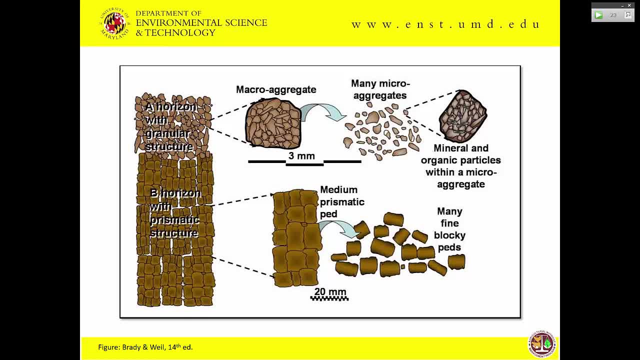 You have a lot of like rounded stuff- They call this granular Types of structure- And then you get it kind of held together. Anyone ever pull up like a grass clump and like a whole bunch of soil came with it. That's what we're talking about when we're talking about soil structure. 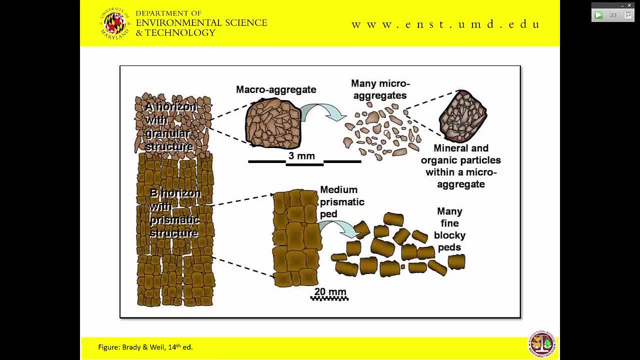 Now, if you have more of these blocky, they call this prismatic structure. Again, depends on your soil types etc. You can get lots of smaller pads. You can get lots of these bigger pads. It depends on kind of what's going on in your soil. 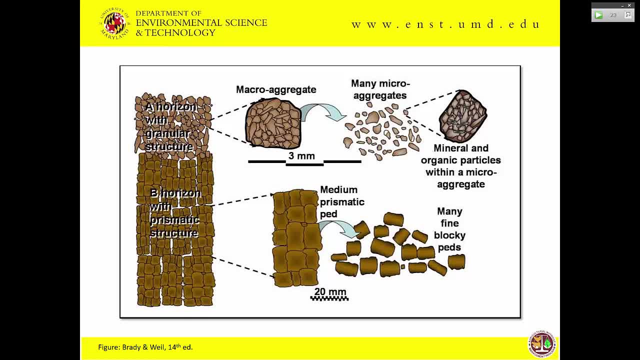 When you pull it up and it crumbles away, Not a good sign. You don't have that great of soil health. You want it to pull up and clump. So we already did this first question: How does organic matter affect the soil texture? 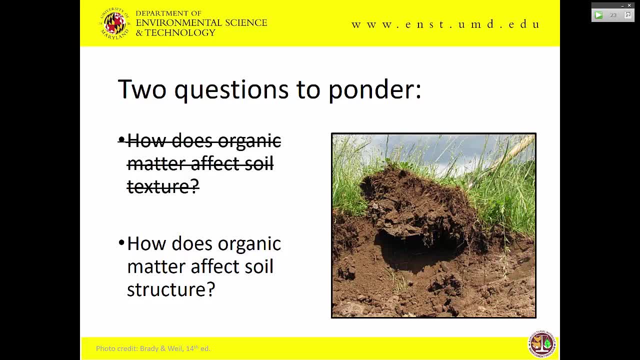 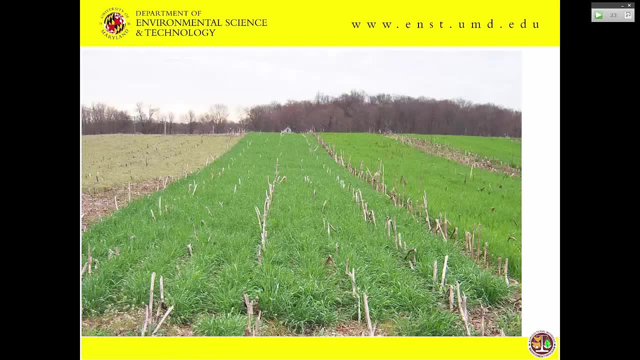 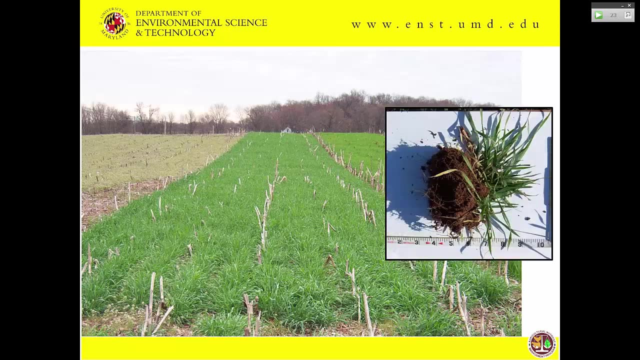 But what about soil structure? How does that impact it? Improve it or decrease it? Improve: Improve Great, So does not impact texture, Does impact structure? To show you, This is just a picture of a again pulled up a clot of soil. 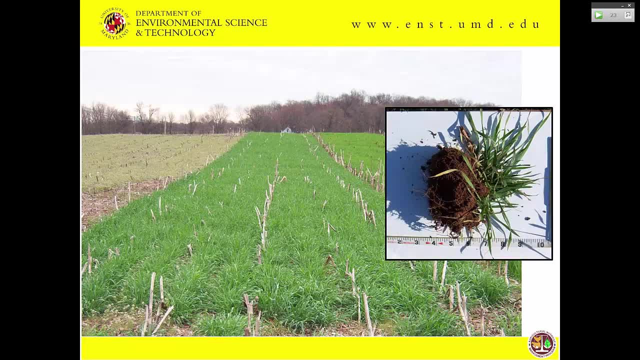 That's what you want. You want to look for those aggregates, Those nice clumps, But keeping your soil in a cover crop- that can certainly help with the soil structure, Growing cover, lots of roots, etc. Can help improve your soil health. 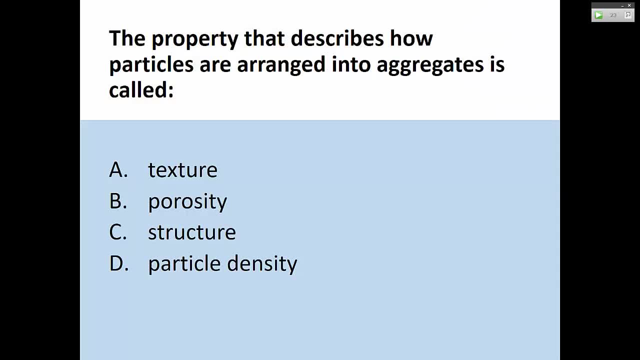 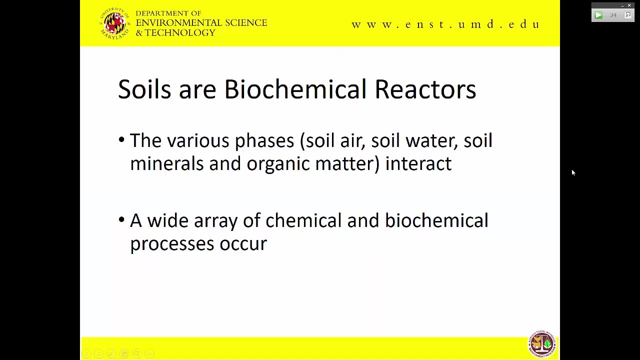 So again, review Properties. that describes how particles are arranged into aggregates. What is that called? All right? Yes, most of you said structure, Nice, We'll talk about particle density coming up, All right. So basic summary of what we just talked about is that soils are essentially biochemical reactors. 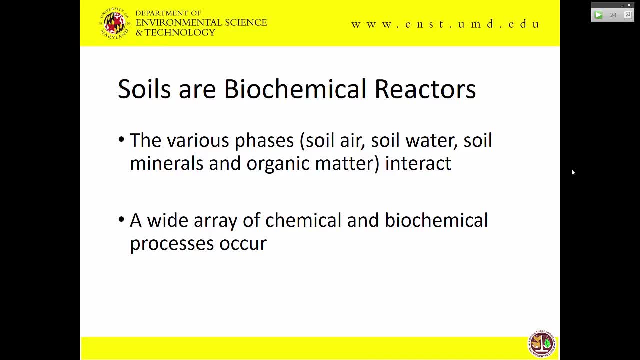 You've got biological stuff going on, You've got chemistry going on, You've got all kinds of stuff And you have to think about how all of these different phases interact A lot of times, for a long time. you know, scientists, we like to, we're kind of reductionists. 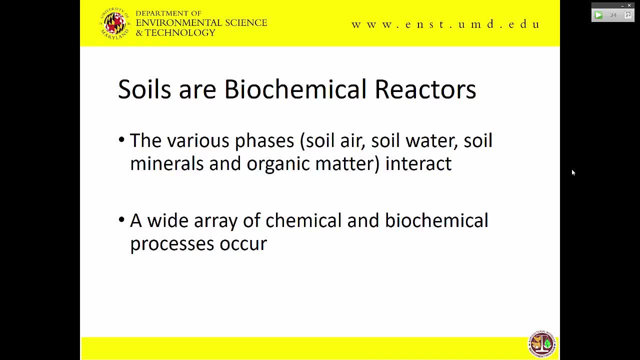 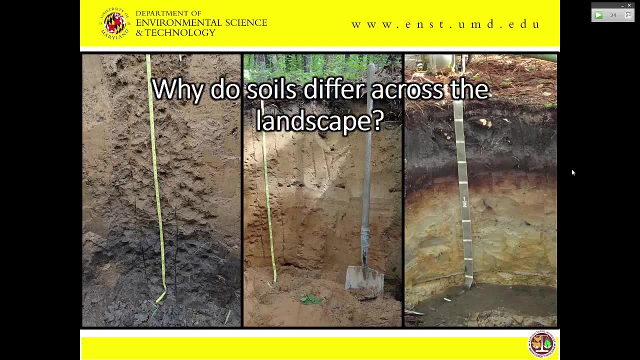 We like to get it down to the smallest parts so we can understand what's happening. But with soil you have to think about the whole picture because there's a lot going on that impacts one another. So now, kind of the next stage is: we've talked about how soil structure is. 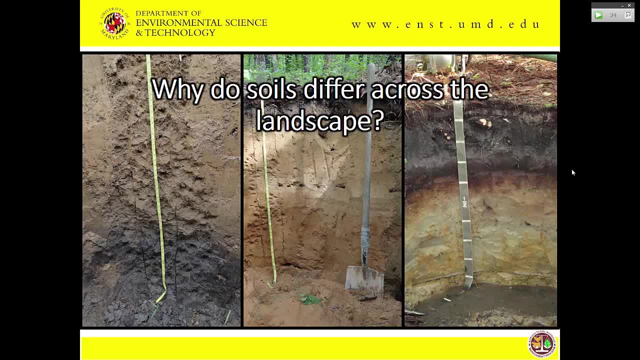 But why do we see these differences in soils as you go across the landscape? Has anyone ever noticed these kinds of things? Some places you have like lots of topsoil, Other places you'll have no topsoil, Like my neighborhood. 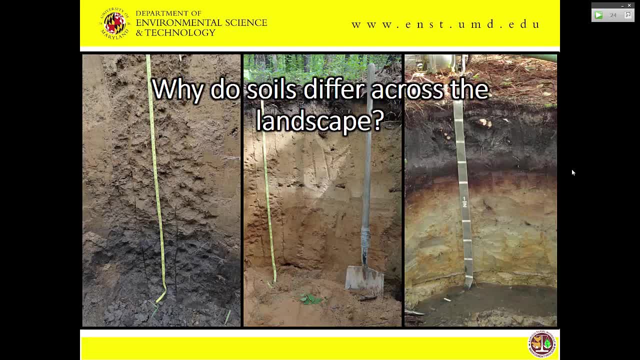 But it does change. Here you can see it's dark the whole way through. Here it's dark and then light and then kind of dark, And here you've got really dark way below. It's kind of crazy to think about. I'm going to tell you why you get this. 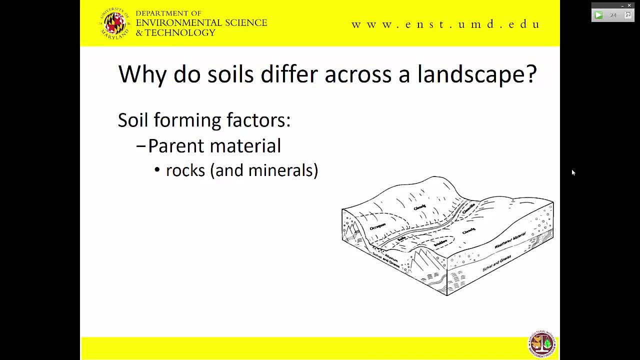 Because we have something called the soil forming factors, And this explains why soils are formed differently across the landscape. So, first off, you've got to think about parent material. That's why I told you about those physiographic provinces, Remember. 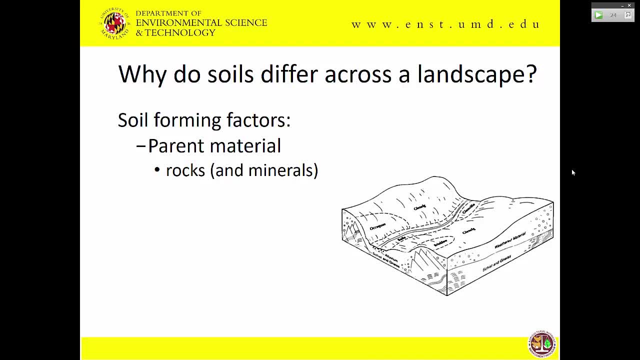 The Atlantic Coastal Plain Most of the rocks are made up of kind of sandy material. That's why you get more sand. The Piedmont tends to have finer textures, like clay rocks and things like that, So when they break up you get more clay. 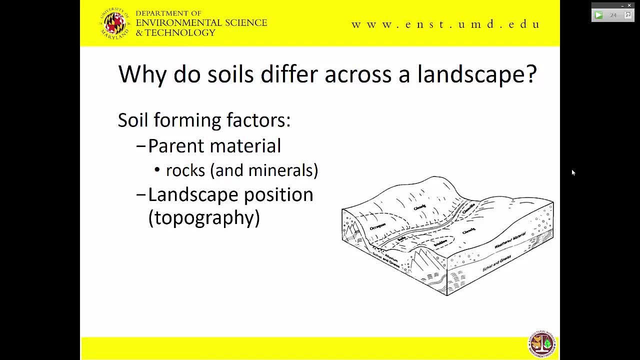 So parent material plays an important role. Landscape position: If you think about you're on the side of a hill, what's going to happen? a lot. What are you going to get? a lot of Runoff and erosion, right, So you're not going to get a lot of topsoil being able to build here if all of it's constantly washed away, right. 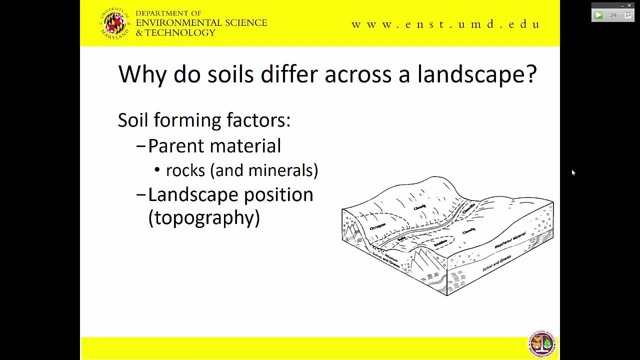 But down in the valley, where all that's collecting, you can get nice thick topsoil, aren't you? That's where all the soil is going to kind of accumulate. So where you're on the landscape matters. Biotic factors. 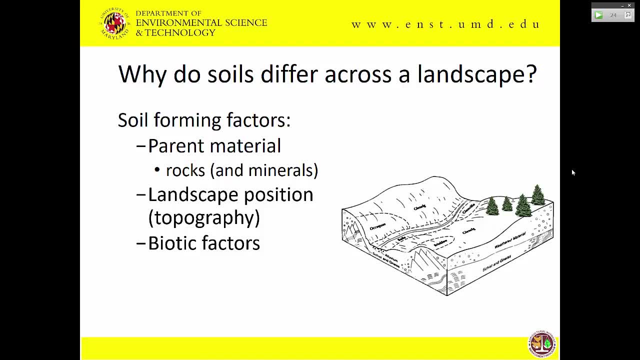 What kind of trees, what kind of animals do you have? Places where they don't have earthworms? Again, I have examples from Minnesota, because that's where I did my graduate work. They, for a long time earthworms weren't in Minnesota because it's too cold up there. 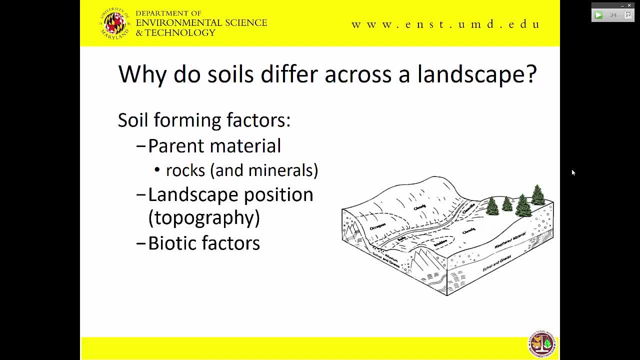 But as it's been getting warmer and as fishermen have been bringing them in for fishing, the earthworms are completely changing the floor landscape. Before you'd have like all these little trees growing up. Now it's only the big trees. 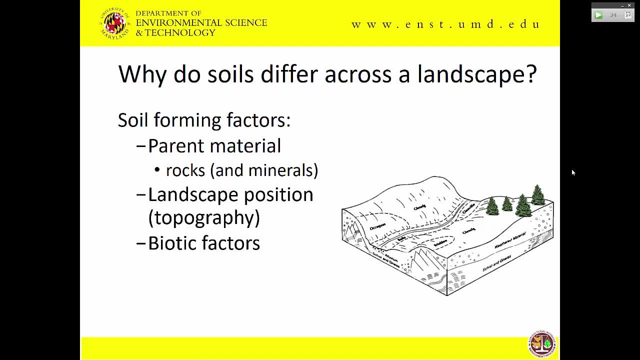 And it's just in the way that the earthworms have changed the soil, which is kind of crazy. So you've got to think about that. Hardwood forests: They don't have a lot of leaves that fall every fall, compared to like a deciduous forest. 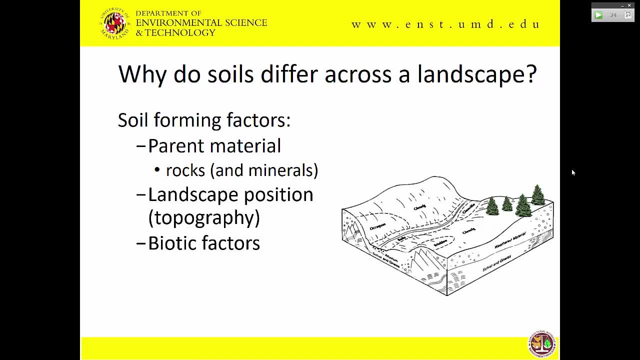 Like we have out here, right? So adding in those leaves, That's going to change what's happening in your soil. All of these things matter. Next is climate. Yeah, the desert where you don't get much rain, Probably not going to get as much nutrient cycling. 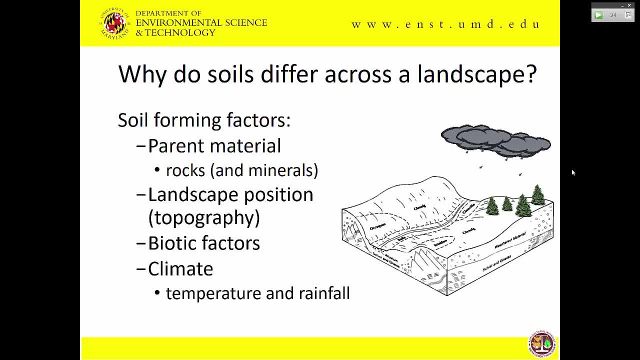 Are you in a cold tundra? You're going to get a lot of organic matter built up there. They have really high organic matter soils but there's not many bacteria that live in those soils to help decompose it because it's so cold. 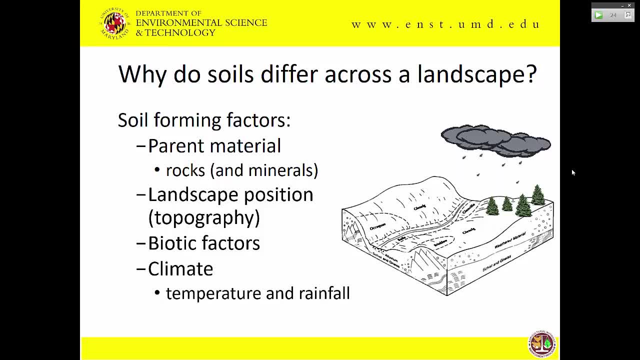 So you get these really thick horizons, A horizons, Topsoil. Is it really wet, Is it really dry, Is it really warm, Is it really cold? All of that also impacts your soils. And then, finally, just old-fashioned time. 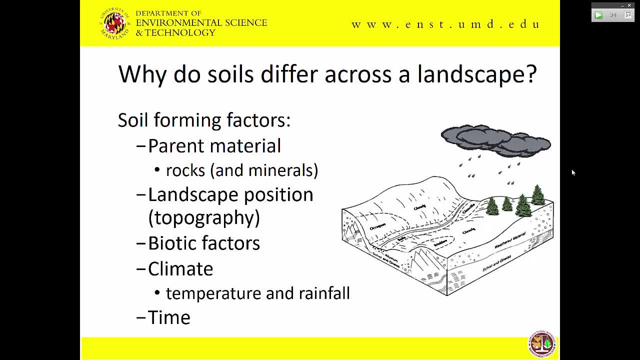 How long has your soil been there Out? where they have really old soils, they don't have much topsoil either, because the bacteria have eaten most of the stuff that they need to eat. Here in Maryland we have those really thin soils that are on the resistant rock. 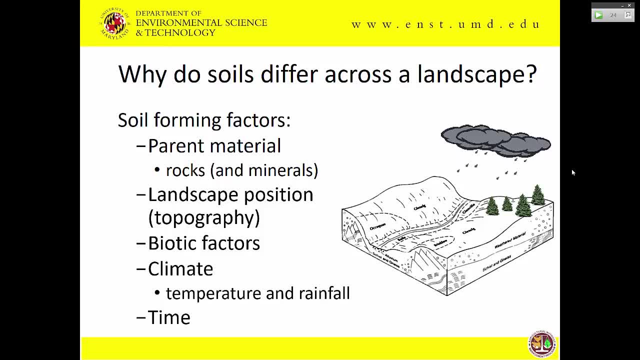 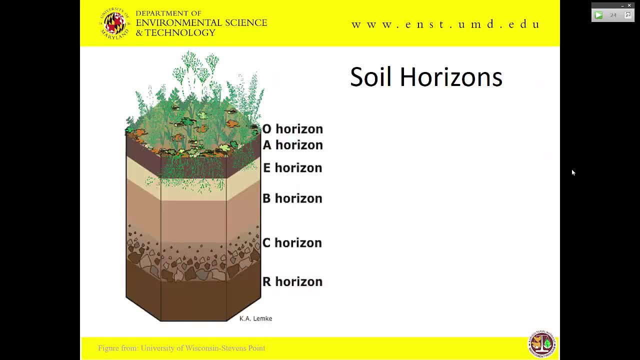 And that's because it's just taken that much time to even produce three feet of soil, So it can take millions of years to form this stuff. So, believe it or not, there are people who study the layers of the soil And again, you might think this is weird, but it's actually kind of cool. 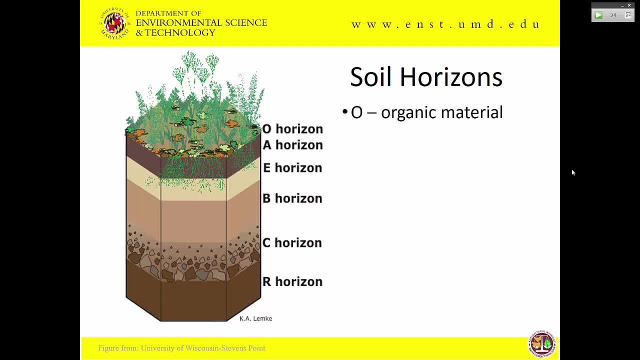 You have the O horizon, which is O for organic material. So if you think of, like those peaks Trish was just talking about, that's an O horizon, That's just organic matter, no minerals. Think of the forest floor, a deciduous forest floor. 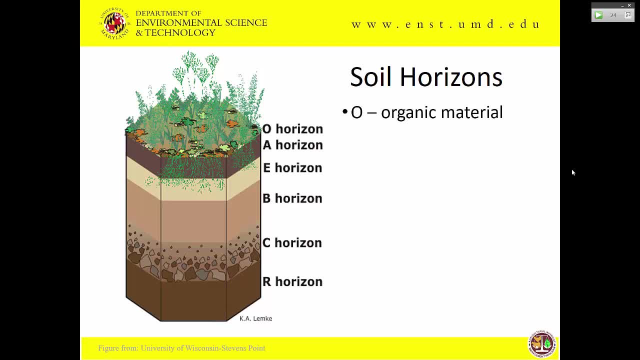 All the leaves on top. that's still considered part of the horizon, but it doesn't have any sand, silt or clay in it, So that's O horizon. A horizon is mixture of the mineral particles and the organic. I think of this as the topsoil. 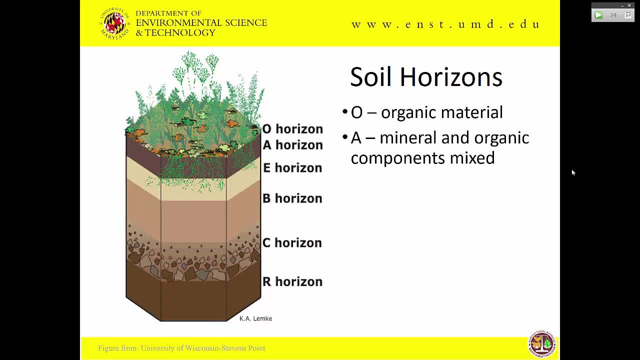 It's usually the nice kind of darker layer right on the top, The E horizon. E is for eluviated, Think of leachate. Leaching Clay is iron, aluminum. have moved out of this area to further down in the profile. 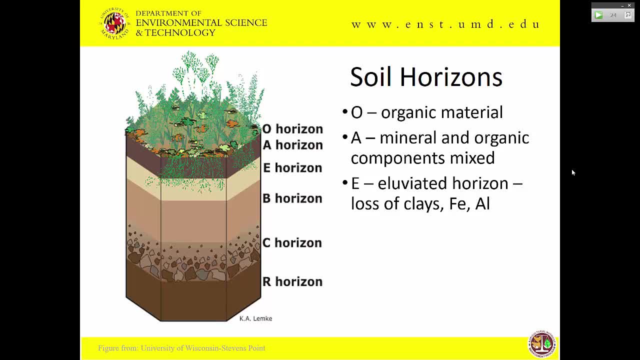 So it's leached out of that area, Leached out, Yep, And it's often kind of light in color. That's what kind of reminds me that stuff has been leached away. It's just lighter in color. You don't have the organic matter, et cetera. 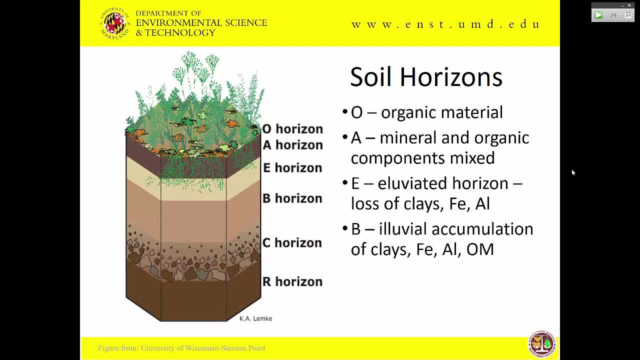 The B horizon is the illuvial, So that's where it's accumulated. E is where it's leached out of, B is where it settles. Kind of think of it that way. So you're going to have higher levels of clays, the iron, the aluminum. 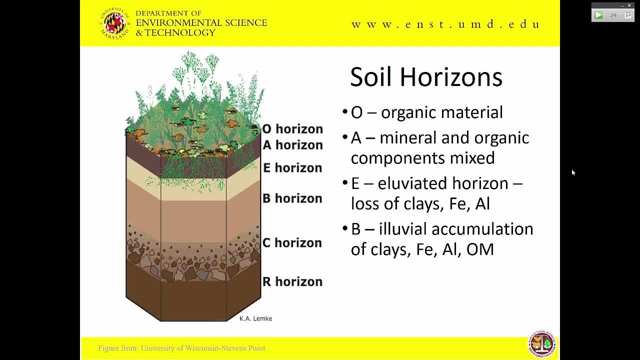 You may have a little bit of organic matter. It's not going to be like the A horizon, though It'll definitely be a distinct color versus the A horizon. C is going to be unconsolidated bedrock. So this is where you find a bunch of chunks of the bedrock at. 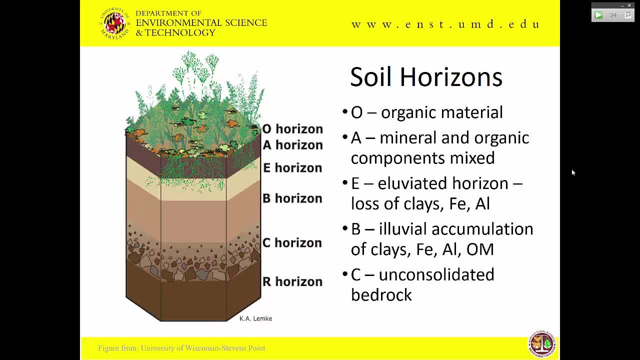 It's where it's starting to turn into the soil, but not quite there yet. And then what we call the R horizon is just the hard-fed rock. I don't really know who named these like gave them the A, B, et cetera. 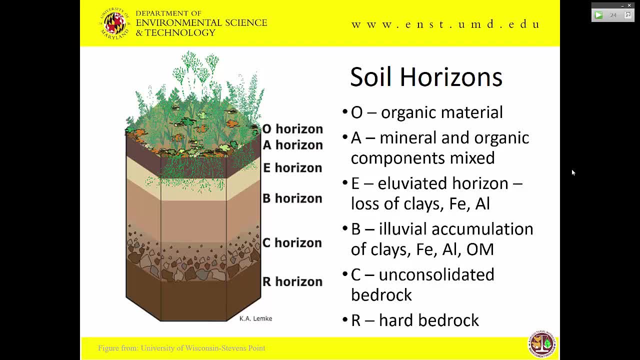 But this is what they are Now. do note: you're not necessarily going to see all of these out in the desert. Do you think you'll have an O horizon? No, So they could go in a bunch of different orders. 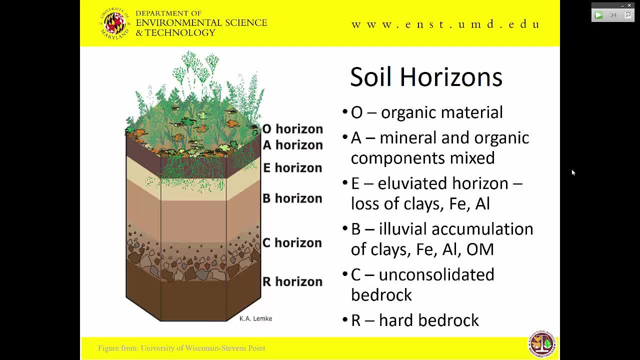 We've even seen- I've seen crazy things where there was an old homestead that had the topsoil, et cetera, And then you went down further and there was another layer of topsoil, So like they had come in at some point and like completely covered the land with topsoil. 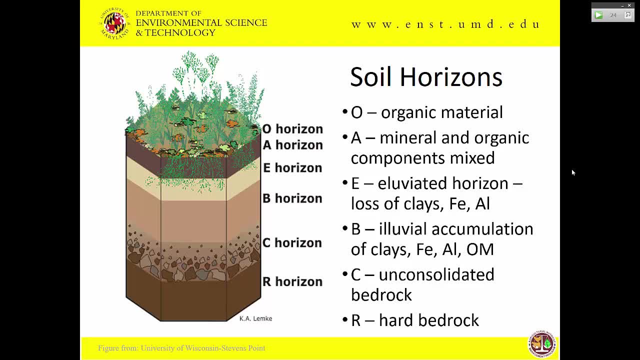 I don't know if they were trying to level it out or whatnot, but you could actually see the different levels in the soil. So you could see history in the soil. I know I'm a toad and herd, but let's give you an example. 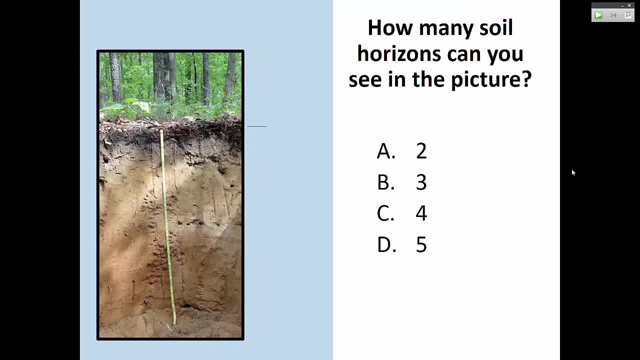 How many soil horizons do you think you see in this picture? I expected this one to be a little more all over the board. Most people thought four, or, sorry, five, because it's D. Some people picked answer five, which is nothing. 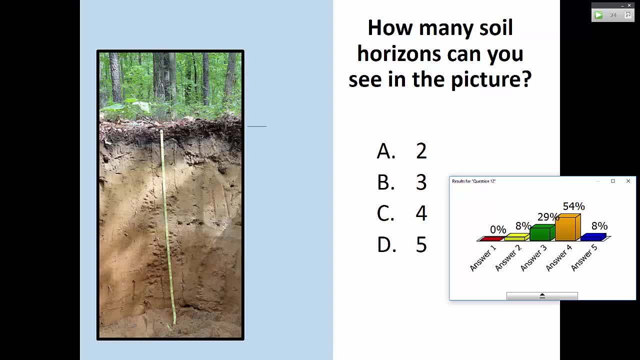 But that's okay, So there's. oh, so some people must have thought six, So let's actually go through this. All right, I see an O horizon Forest. right, So you got the leaf litter at the top. 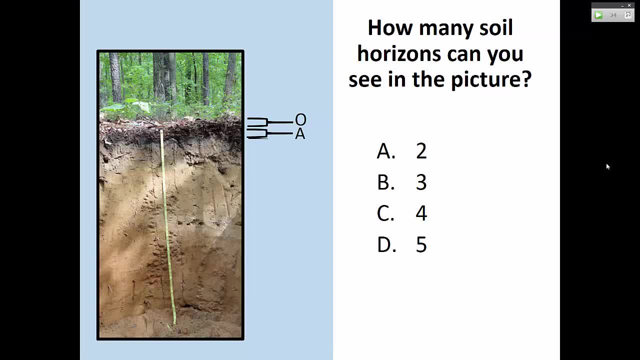 You got the topsoil, So that's the dark stuff. See how it's a little lighter here. I'd call that an E. That's where you saw some stuff leached out. And then there's one B layer. The next one isn't unconsolidated. 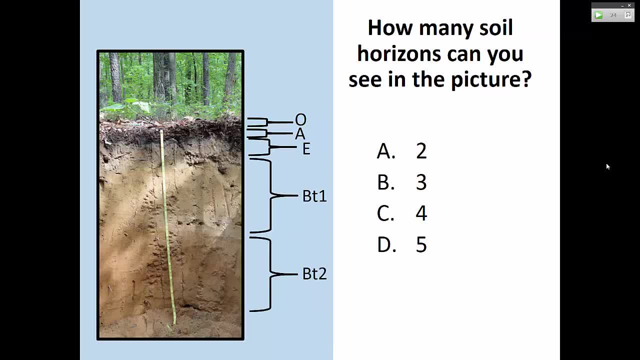 Bedrock though. So there's actually a second B layer. I know Soil scientists are crazy And then technically you could go further beyond that, But this is what they call the soil horizons. They actually have teams. 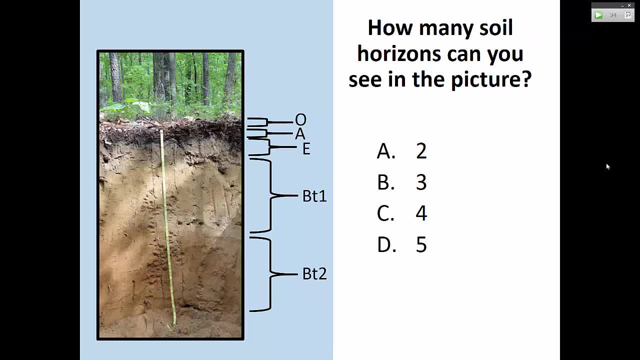 I don't know, Did anyone go to University of Maryland be on the soil judging team? They just won. this past year They won the national championships. So there are people that actually go around and judge these things And they're quite good. 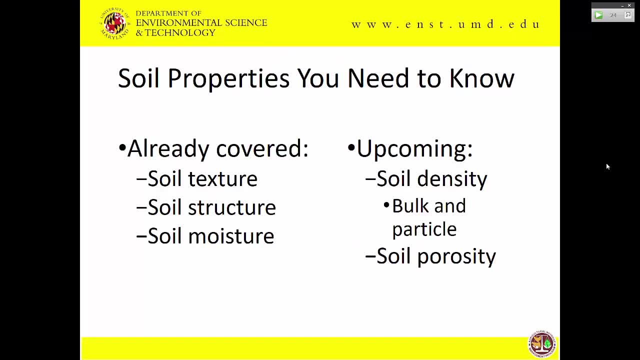 I was not on the soil judging team, So All right. So a couple things you need to know. We talked about structure, We talked about texture And we talked about moisture. Right, Know those. The other ones that don't fit into my fancy story are soil density and soil porosity. 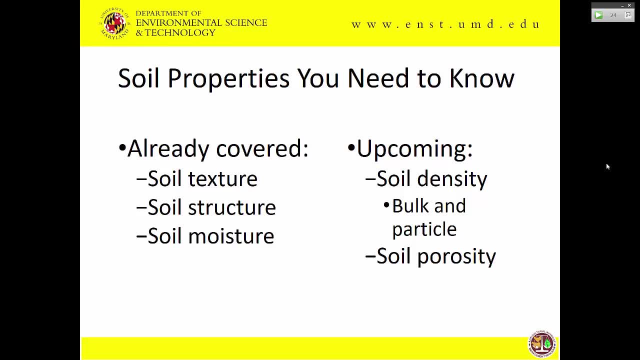 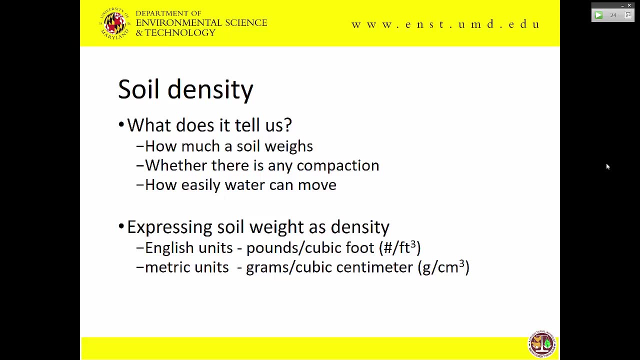 So we're going to talk about those next. Density comes in two forms: Bulk and particle. The reason why we care about the density is because it tells us, kind of like, how much the soil weighs and how much pore space it has. So you can get a good idea of if you have compaction. 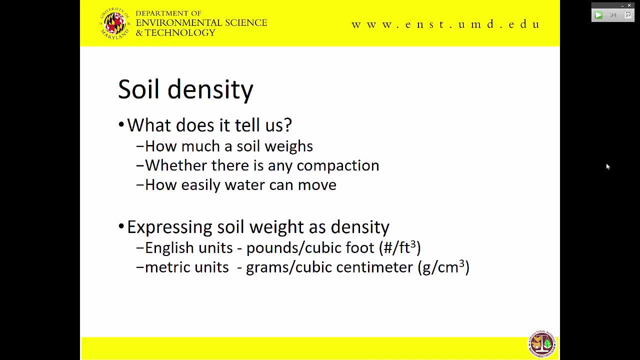 Also, it tells you how easily water can move, Because you know if you have a sandy soil it can move pretty quickly, But a sandy, compacted soil, it still won't move quite as fast. So you need to understand the difference. 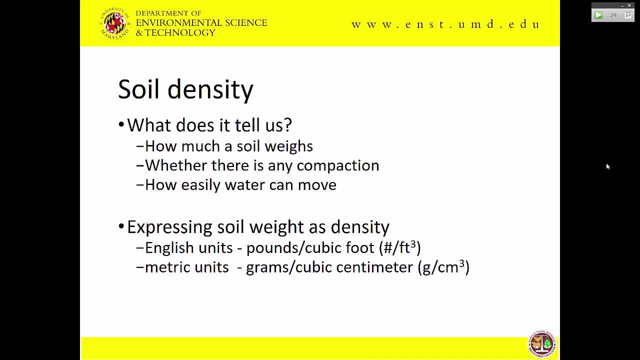 So we usually we'll talk about a couple different weights. Here in the US you might see it as pounds per cubic foot. Scientists typically use large weights, Or British- you know not British. you use metric units, So we'll talk about it in grams per centimeter cubed. 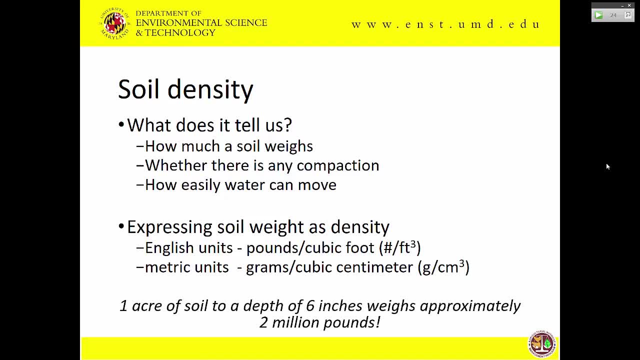 Interestingly, on average one acre of soil just to a depth of six inches, if you can kind of imagine that spatially, that weighs two million pounds if you consider like the average bulk density of a soil. So again kind of gives you an idea of you have to think about that in regards to like. 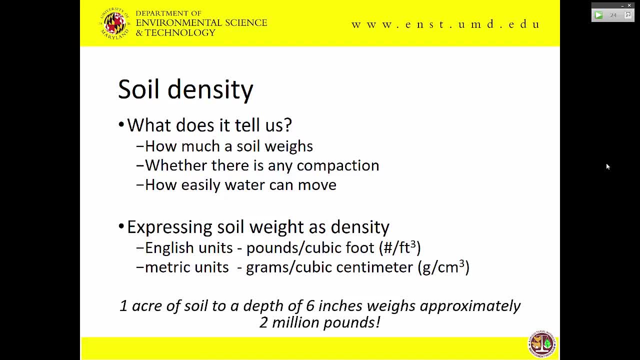 plowing the soil Right. If you're going to a depth of six inches, you've got to be moving, moving through six or two million pounds of soil. So it helps think about, you know, no tillage versus tillage, et cetera. 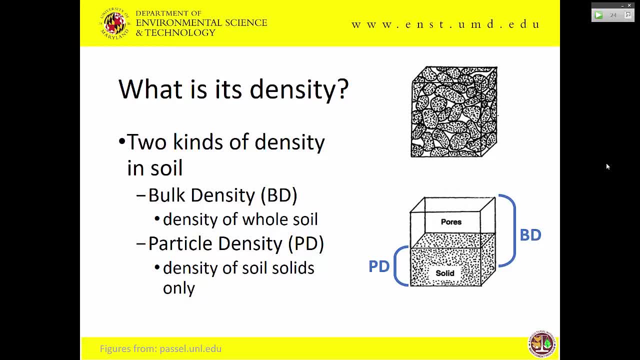 So, like I said, two different types. We have bulk density, We'll refer to it as BD, And then we have particle density or PD. The difference is bulk density would be this whole cubic volume here. It includes the pore space. 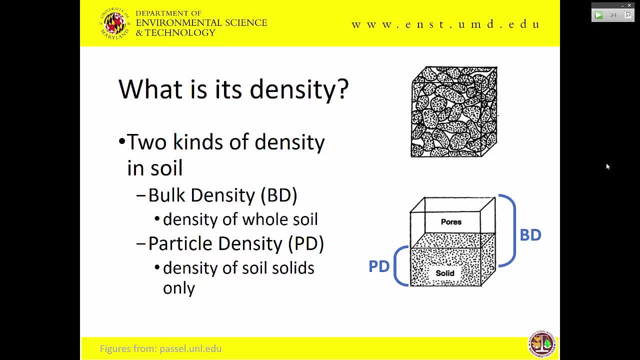 Whereas particle density would only be if you completely crushed all the solid spots into one area. That would only be the cubic area of that smaller volume. Does that make sense? So one, we kind of consider how many poles are inside of it. 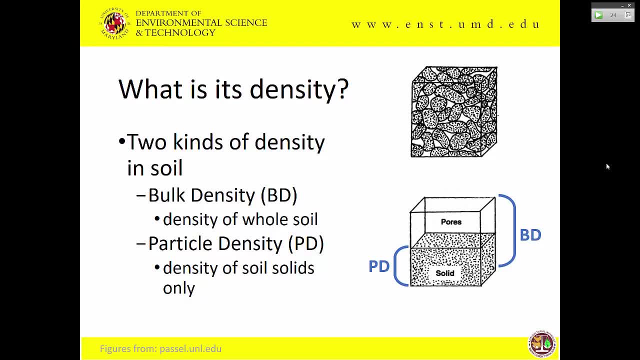 And the other one is only taking into consideration the solids. It doesn't take into consideration the air space in it at all. Now again the reason why we want to know both of these. we usually only talk about bulk density, But if you want to figure out how much pore space you have, you want to know the particle. 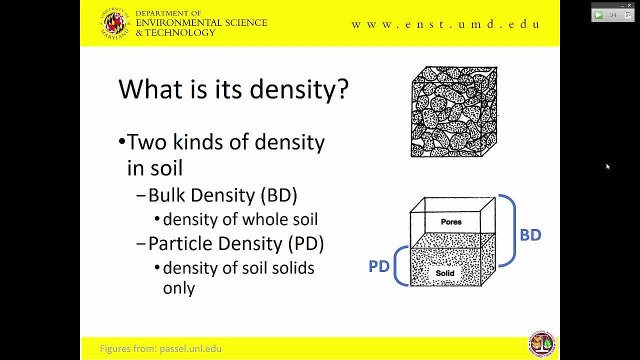 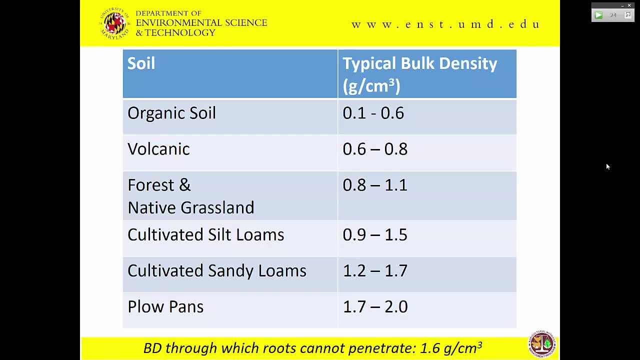 density as well, Because if you subtract two you get the pore space. So typical bulk densities There's organic soils, usually pretty light and fluffy, Lots of pore space, Not a lot of solids, So the bulk density is going to be small. 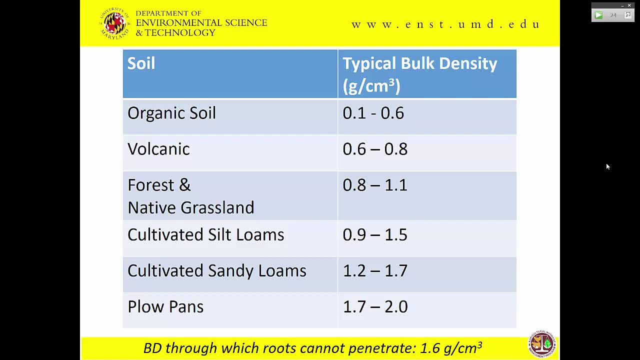 Volcanic soils- again kind of fluffy Forest- and native grasslands will range from 0.8 to 1.1.. Cultivated silt loams will be 0.9 to 1.5.. Cultivated sandy loams will be 1.2 to 1.7.. 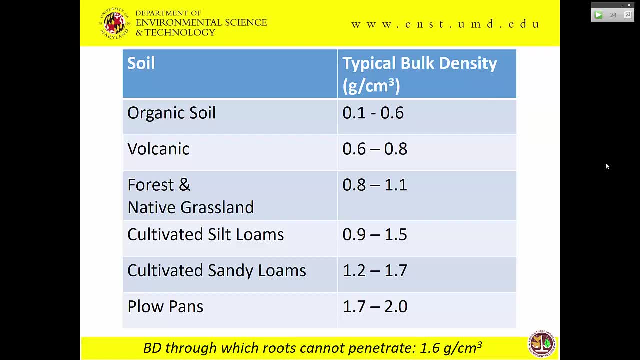 Now, a plow pan, which is what we get sometimes, is usually from 1.7 to 2.. And the thing is that plants- plant roots- really won't go through anything above 1.6.. So plant roots do not like bulk densities higher than 1.6. 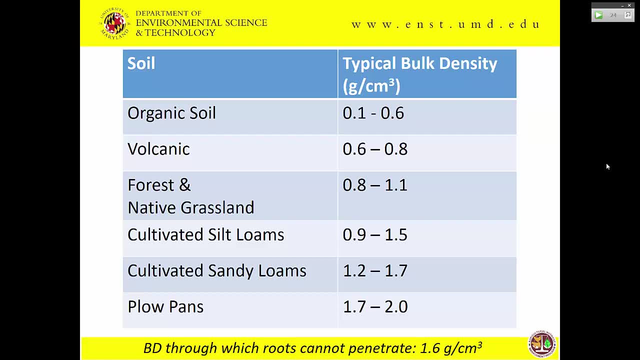 And that's why you get plow pans right. You have that heavy equipment going over the field but you do plow whatever the top six to eight inches, And that's so. you get compaction below that but you get nice and fluffy soil above that. 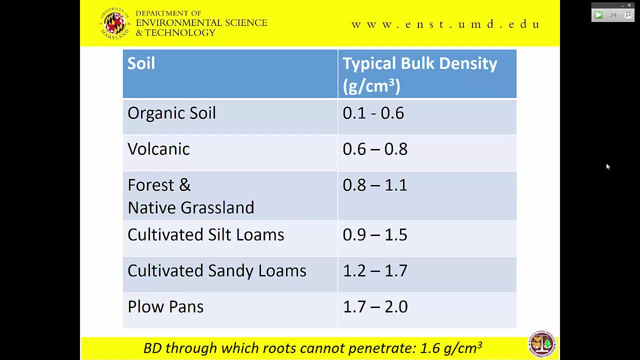 That's unfortunately what happens with these plants. Is there a way to measure that? What's that? Is there a way to measure that? Yes, Yeah, we're going to talk about that, Okay, And you're going to practice too. 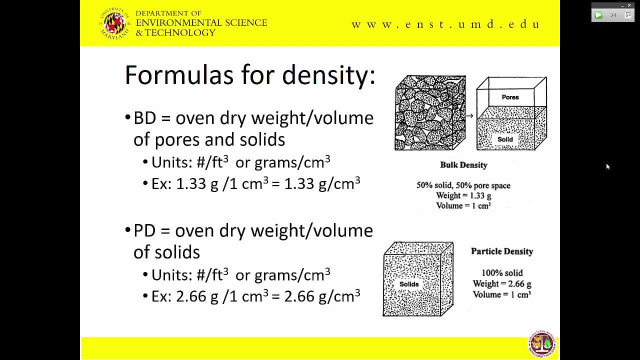 Okay. So formulas: Bulk density is the oven-dry weight divided by the volume of the pores and solids. So essentially like, if you pull up one of these, Okay, If you pull up one of these clads of the soil, you'd have to try to figure out the volume of it. 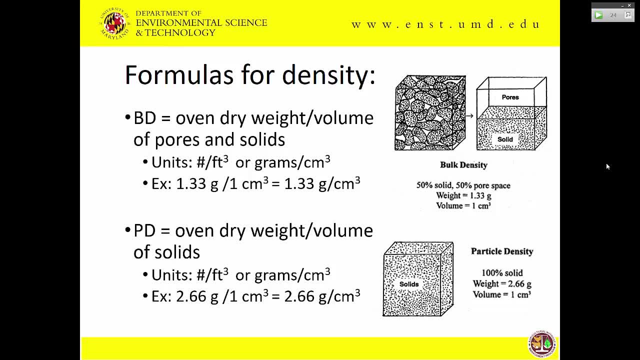 And then you figure out the oven-dry weight of that soil and you can figure out bulk density. Scientifically, what we do is we have rings- metal rings- that you pound into the ground, pull up the soil and then you 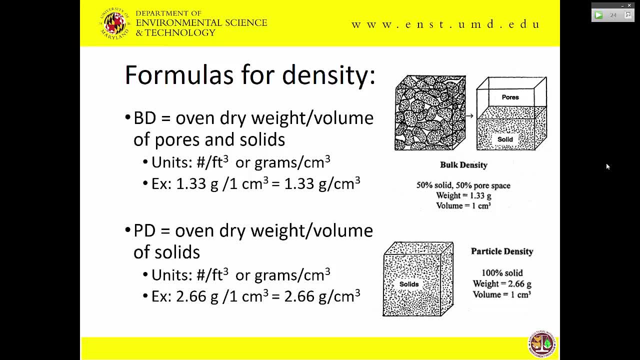 So you know the volume- It's a known volume- And then you dry it out, figure out what the dry weight is and you can figure out bulk density from there. You don't have to worry about trying not to crush the soil deeper than it would be. but 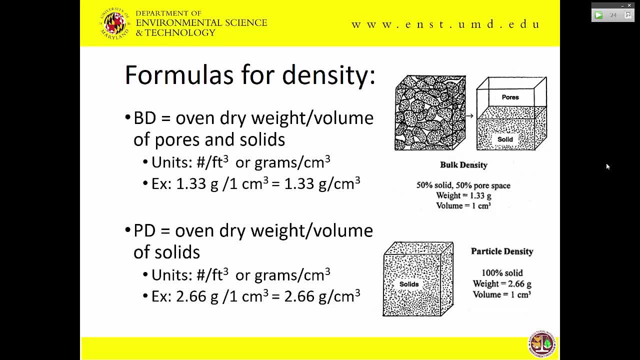 So this example- I think we- I caught a mistake that I made. I think it says one in your printouts but it is 1.33.. Just caught that after we printed these. So say, in this example the soil is 50% solid, 50% soil space, but the weight is 1.33 grams. 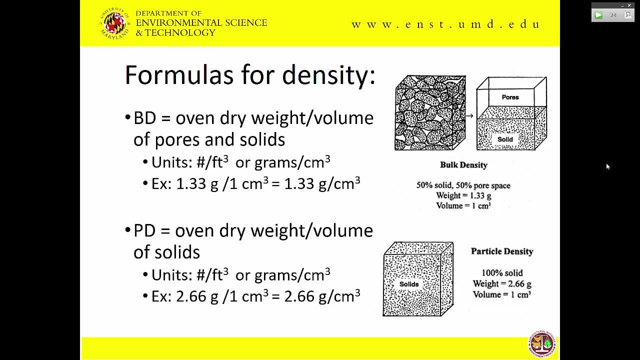 And we know the volume is one cubic centimeter. So 1.33 grams divided by one cubic centimeter equals 1.33 grams per cubic centimeter. Does that make sense? Particle density, again, is a little more abstract to me because it is harder to figure out. 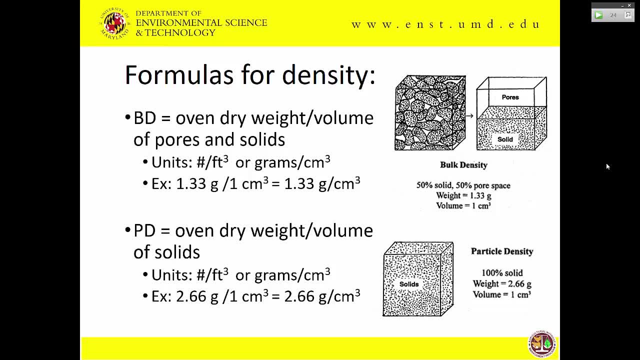 But this one is the oven dry weight divided by just the volume of the solids. So imagine that we had just a solid rock that was one cubic centimeter, The weight of it is 2.66 grams and the volume is the same as above. 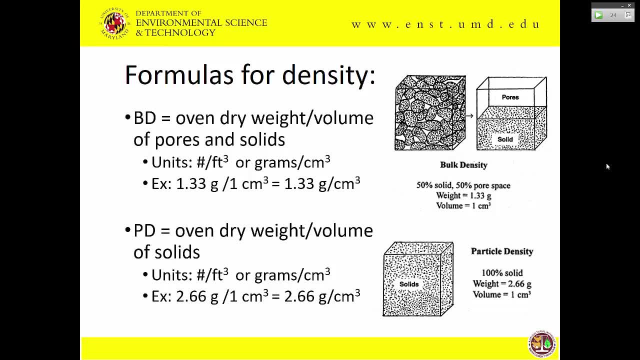 So then, that would be 2.66 divided by one, which equals 2.66.. So, obviously, would plant roots be able to go Through a solid rock? No, definitely not. Would they be good for this one, though the soil up here? 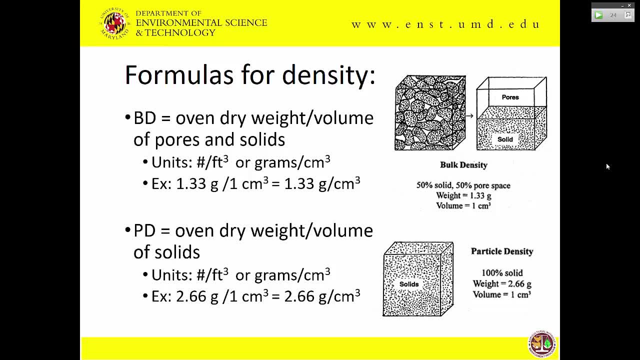 1.33? Plant roots go through that. Yeah, Like I said, particle density is hard to figure out. What you have to do is you basically have to do displacement. So you put some water in a jar, put your cloth in it, see how much water gets taken off. 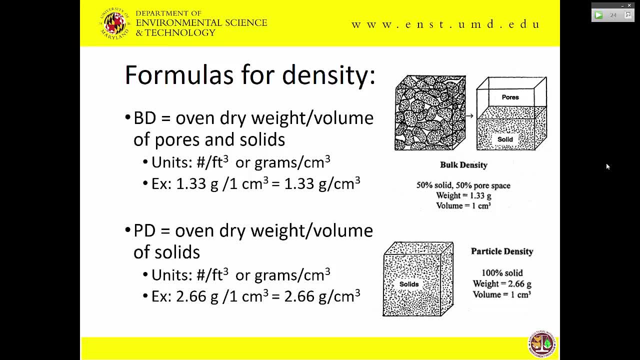 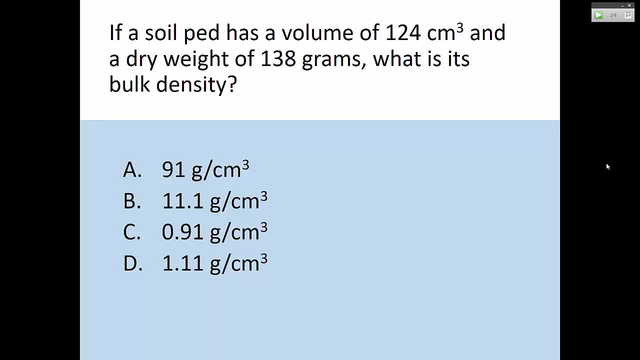 Or thrown off the side and it gives you the volume of the particles. Like I said, it's a little more, a little harder to do than bulk density, So let's practice. Soil pet is the volume of 124 centimeters cubed and a dry weight of 138. 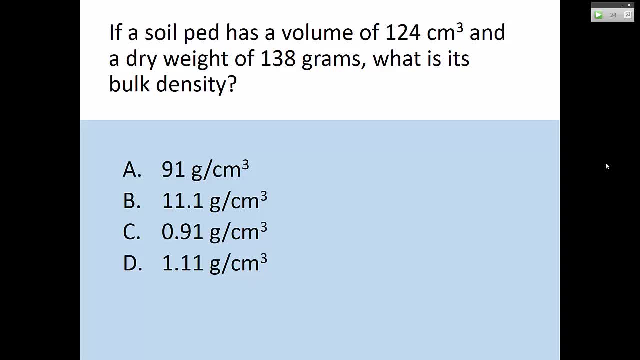 What is the bulk density? All right, let's see. Most people said 1.11 grams. Let's walk through it: 138 divided by 124 equals 1.11.. Good, So you got it. So again, if you have questions, come talk to us about this afterwards. 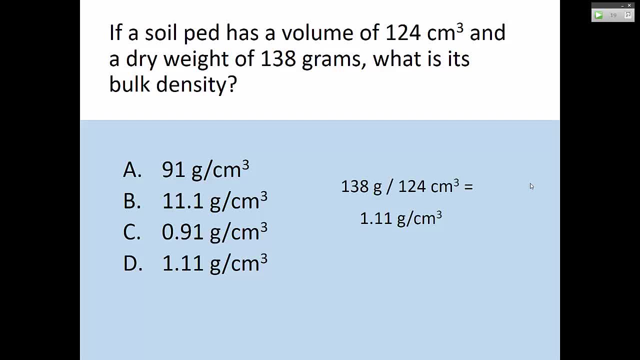 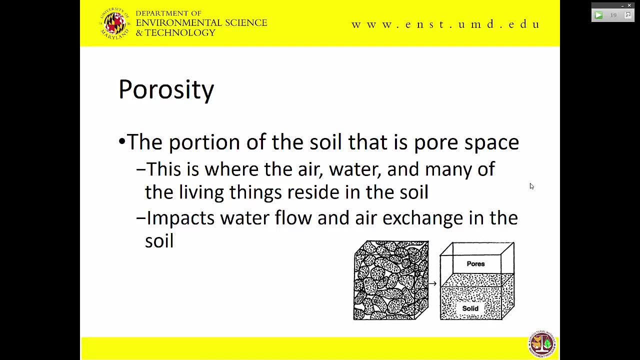 This is something that you could be asked on the exam. All right, porosity, It's kind of the opposite of particle density, It's the volume of pore space. So just this area. You can't take it off. You can't take the top if you were to crush all the solids down. 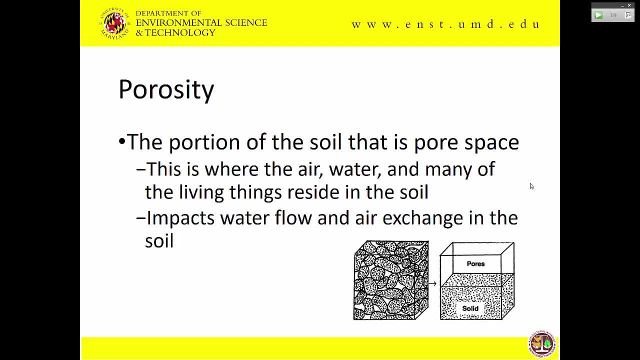 Again, it's importance is where everything lives. It's where the soil and air is, and we want to know how these things can move. So pore space is probably a little more important to know than particle density is, but you need one to figure out the other. 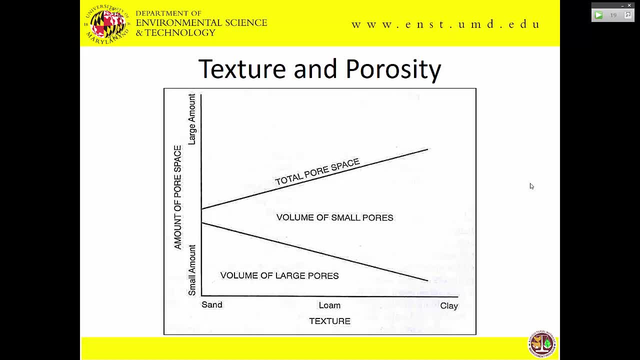 So how this is impacted by texture. Again we have the coarser textures over here. The clays, et cetera are more on the left. The volume of the large pores will decrease. So again you have bigger pores with the sands. 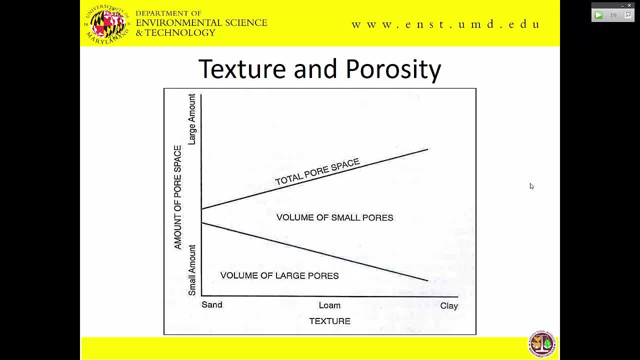 You're going to have less of those with the clays. The volume of the small pores, though, will increase. You have fewer of the large pores in clay, but more of the small pores, So this one, the volume of large pores- is decreasing. 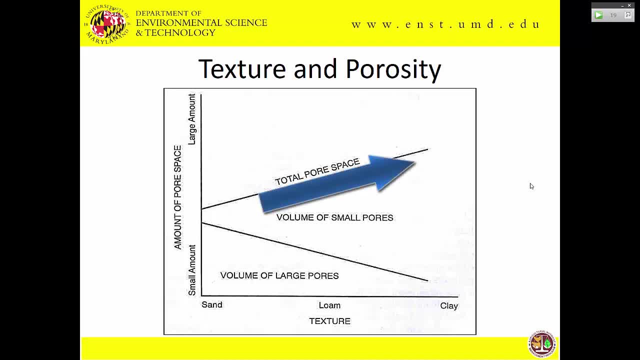 Volume of the small pores is increasing, But the total pore space also increases. And again we talked about that with that clay and we saw that visual. The same amount of water had been added to the sand and the clay, but it traveled much. 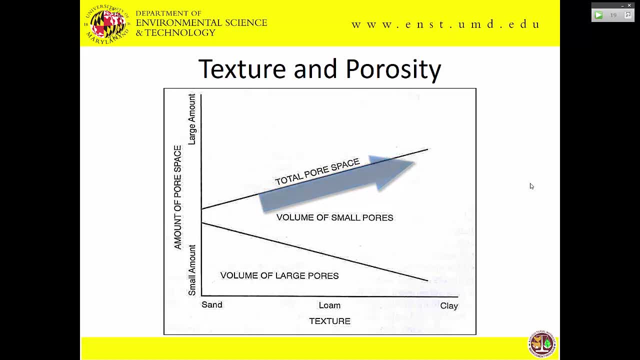 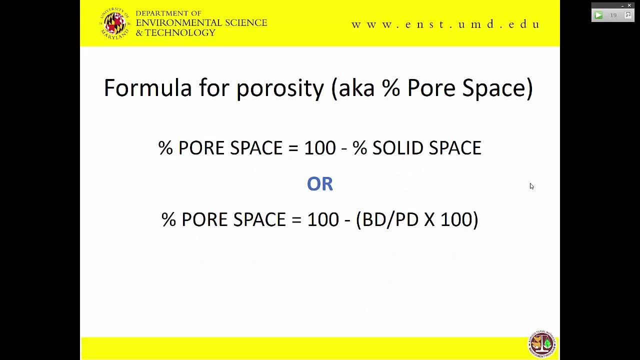 faster, It traveled much less further in the clay. So porosity is actually going to be 100% minus the percent solid space. How do you figure out the solid space? Take the bulk density, divide it by the particle density and multiply it by 100. 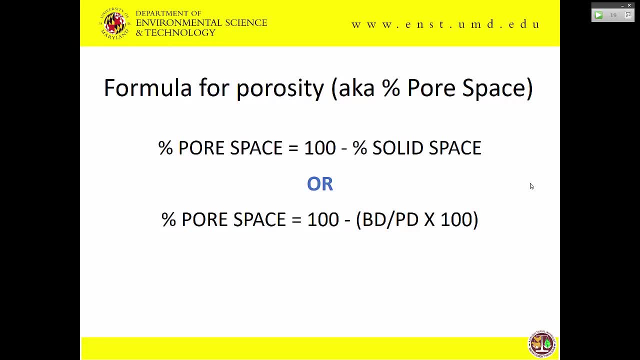 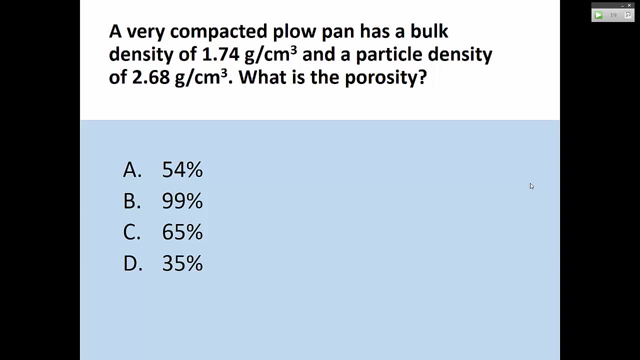 Then take that number, take 100 minus that number. You guys ready to practice this one? Okay, I'm getting blank stares, so we'll move on. A very compacted plow pan has a bulk density of 1.74 and a particle density of 2.68. 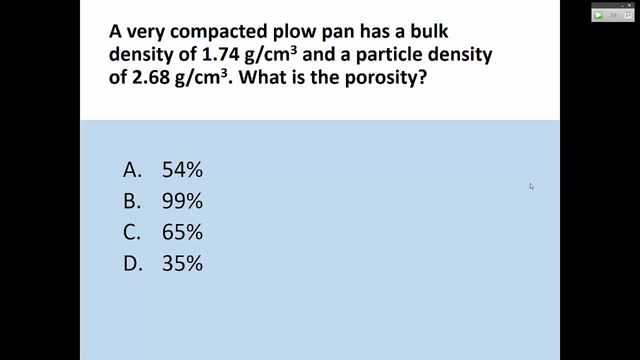 What is the porosity? All right, Only about half of you got answers in and it was all over the board, but most people said answer four, So let's walk through it. This is the formula 100 minus the bulk density divided by the particle density times 100. 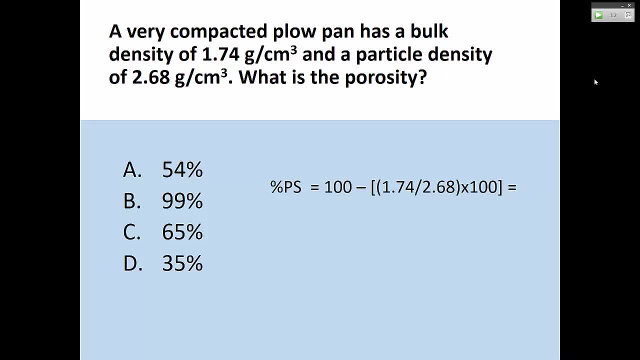 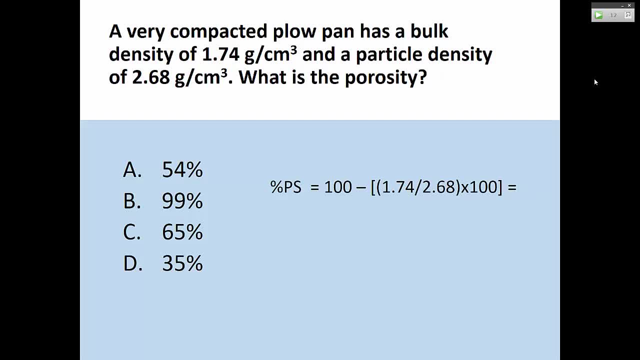 This is the formula 100 minus the bulk density divided by the particle density times 100.. This is the formula 100 minus the bulk density divided by the particle density times 100.. So 1.74 was the bulk density, 2.68 was the particle density. 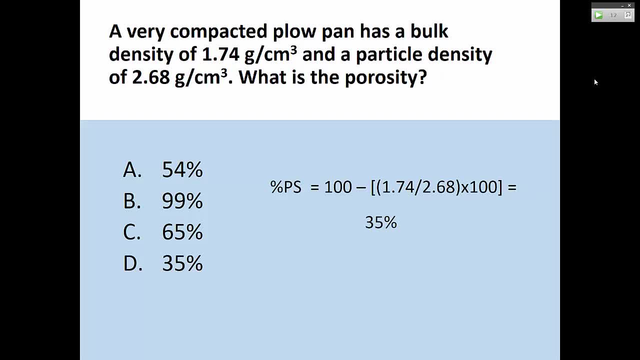 Got 35 percent, So at least the majority who answered, you get the 35 percent, which is good. But remember: BD minus PD: It's in alphabetical order. Or BD divided by PD, I think is in alphabetical order. 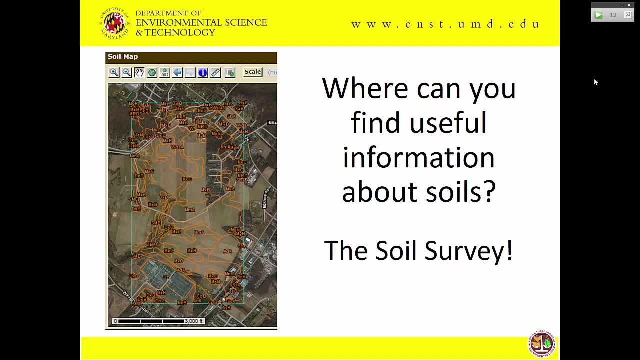 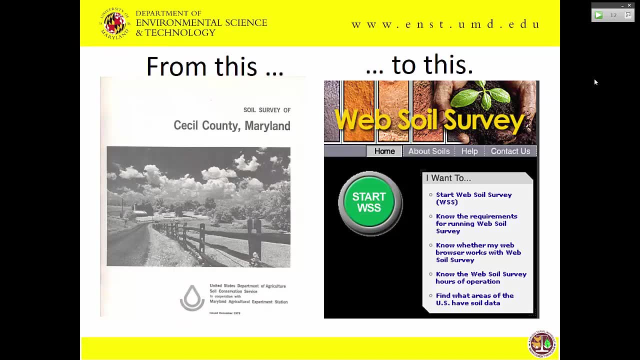 All right. So the last thing I'm going to talk about quickly is the soil survey. The soil survey is where you can find information about the soils, overall soil size and the. the soil was on a particular farm And it was old school For a long time we had. 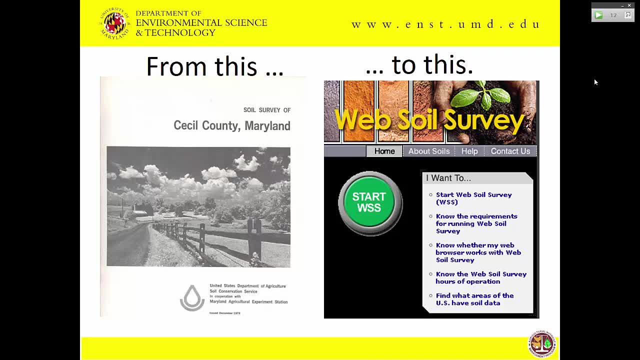 these printed books that went to every county. It took a long time to get them updated at every county, but now they've gone to the internet and you can actually access this whenever you want, as long as you have an internet connection. The cool thing is they can actually update things. I actually we found an. 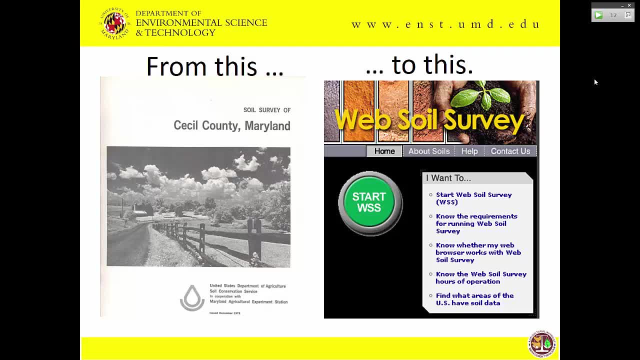 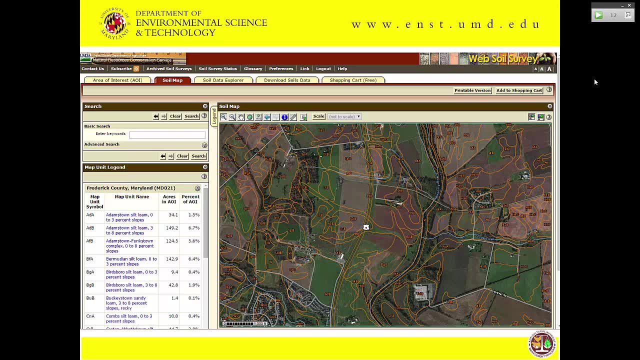 error and I talked to the soil conservation district person and they updated it within a few days. It was pretty awesome. So this is what it looks like. Here you can actually get to the point where you see this different soil maps in here. It will show you if you like, outline an area. it'll show you what. 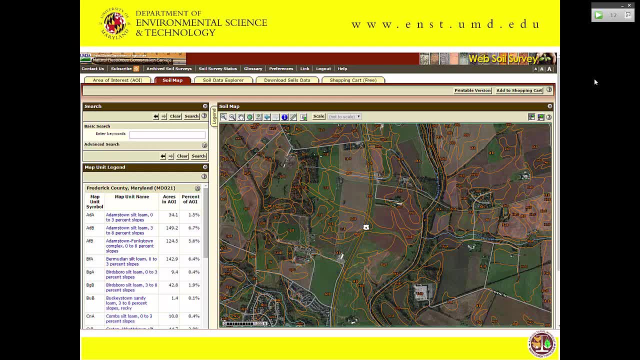 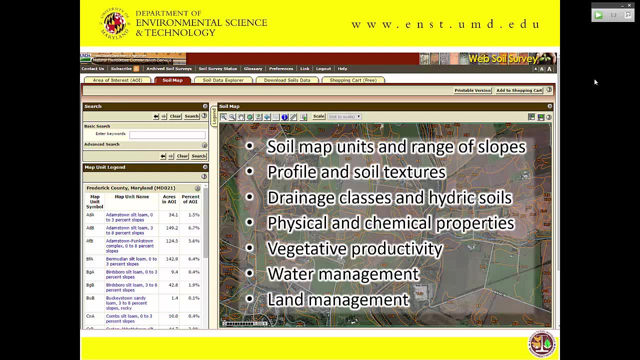 percentage of the soils make up the outlined area that you have, So you can actually see what's the dominant soil in your area, etc. You can get all kinds of information, not only the soil maps and textures. You can get like all kinds of 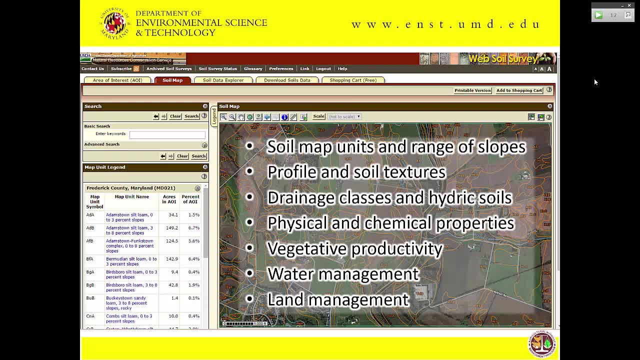 engineering things If you don't know, like how water will move, hydraulic conductivity- Yeah. what's going on with drainage classes and hydro soils, just like any kind of information that can be tied to soils? you can actually find here A lot of it you won't actually need to access. 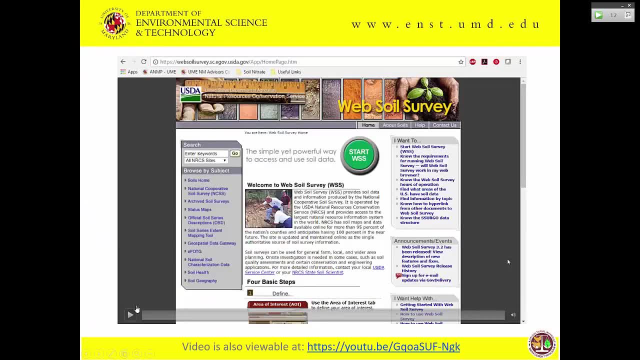 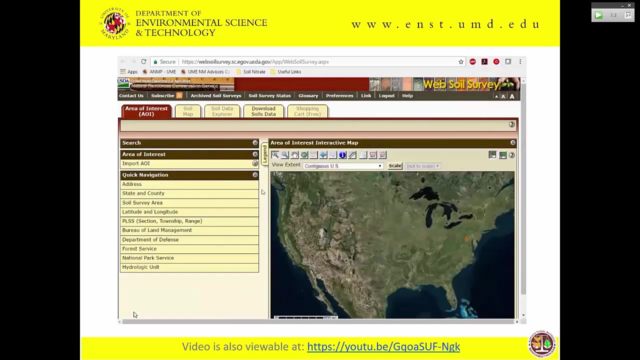 but you can find some important information for land. Today I'd like to demonstrate the Web Soil Survey, a website and program that is operated by the USDA Natural Resources Conservation Service. Once on the website, to get started, you will click on the green Start WSS button. 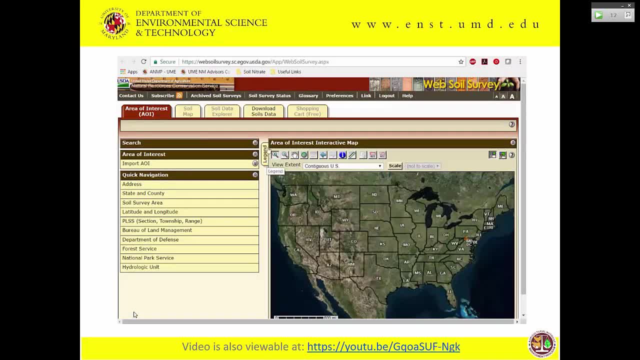 Once the program is loaded, you will see an interactive map of the continental United States, and then you can search for your property in a variety of different ways. One of the easiest ways is to search for the address. In this example, I'm going to look for the Western Maryland Research and Education Center. 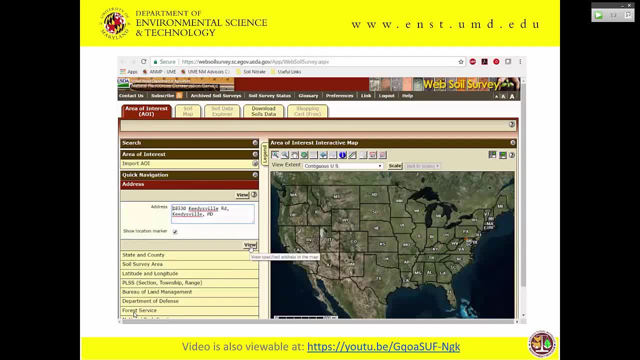 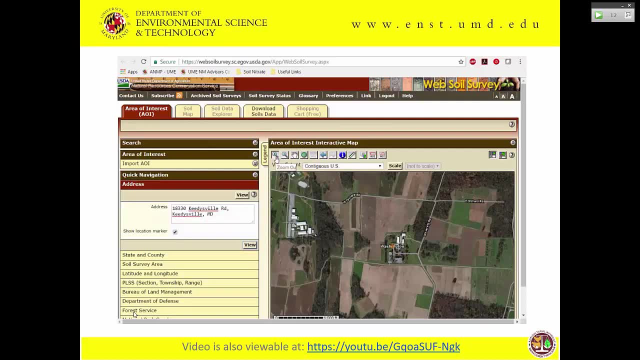 in Keenysville. Once you type in your address, click on View. Now you'll be able to use a variety of tools to either zoom in or zoom out of the map. In this case, I'm going to zoom in a little further. 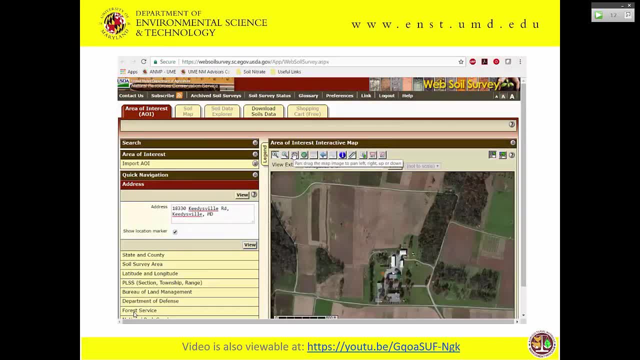 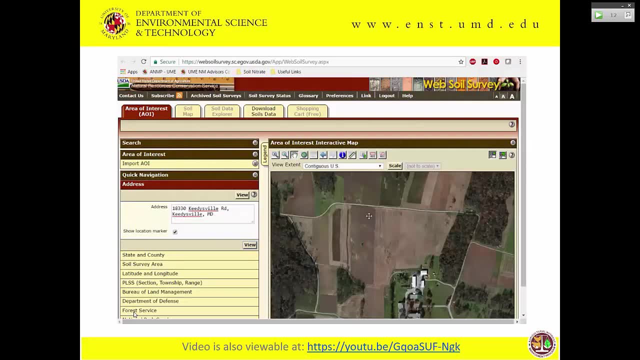 If you'd like to recenter the map, but not zoom in or out, you can click on the Pan button and drag the map. Now, once you find your field, you won't need to tell the program where the field is, So you'll use what's called an AOI, or Area of Interest.